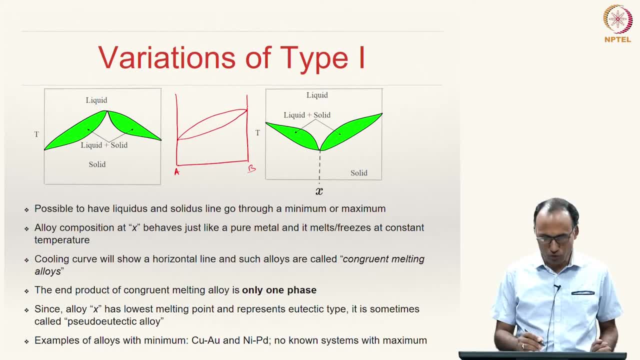 that The isomorphous alloys of the kind that we have looked at so far are looking like that. So A and B are completely soluble both in liquid state as well as solid state. Now is it possible to have a maxima or a minima for this liquidus and solidus line, That is, 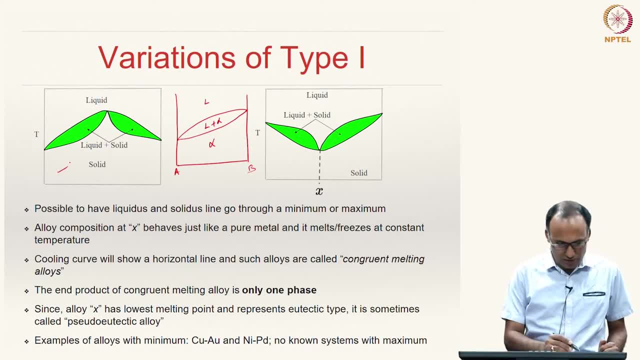 the. if we have something like that, as we have shown here, you can see that this is also an isomorphous. this left side is also an isomorphous alloy, where the liquidus line has a maxima On the right hand side. here you have an isomorphous alloy, So you can see that this is also an 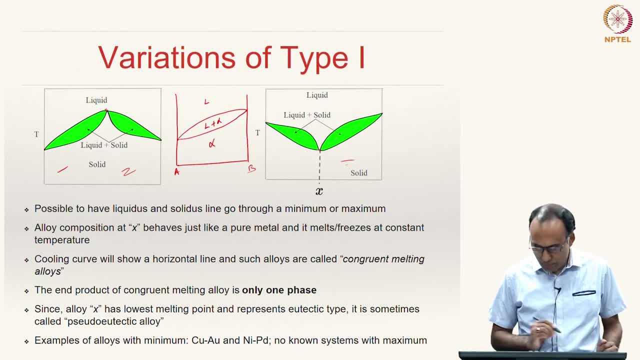 isomorphous. this left side is also an isomorphous alloy where the liquidus line has a maxima. At the right hand side you have a solidus line showing a minima here. So alloys of this kind are also possible. But the alloy composition, for instance, if you look at the 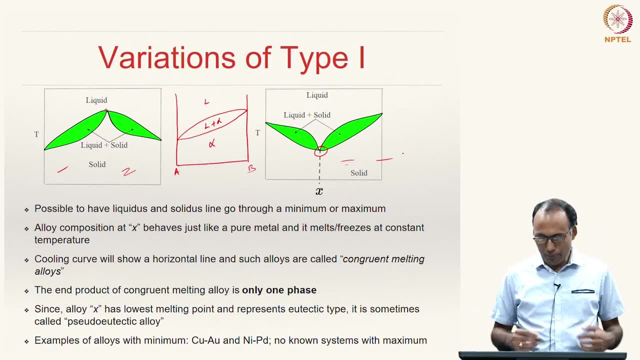 isomorphous alloy variations with a minima that is shown on the right hand side, We see that the composition at x. Let us say you are looking at the x-composition, Then you can see that. So, for instance, let us now compare the solidification of the alloy x. 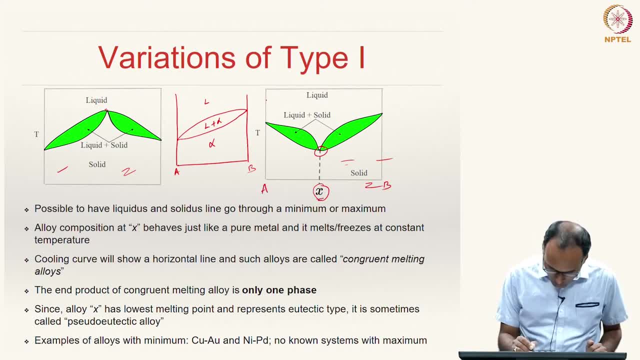 with solidification on A and B Here, when you are solidifying from the liquid state and the A solidifies at constant temperature, right just above this temperature, it is liquid. just below that temperature it is solid. The solidification happens at constant temperature. 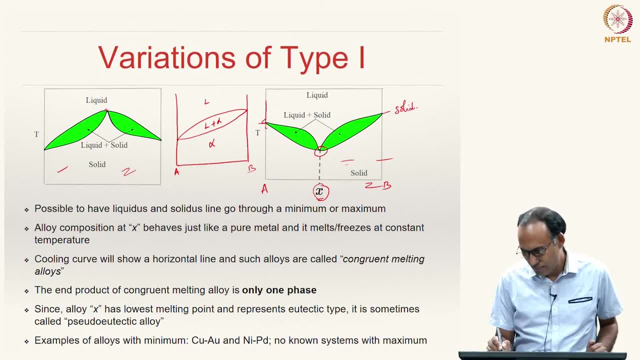 for A as well as B, the solidification at constant temperature, Whereas for all other alloys the solidification happens over a range. for any alloy other alloy combination, for any isomorphous alloy, the solidification starts at one temperature and ends at another. 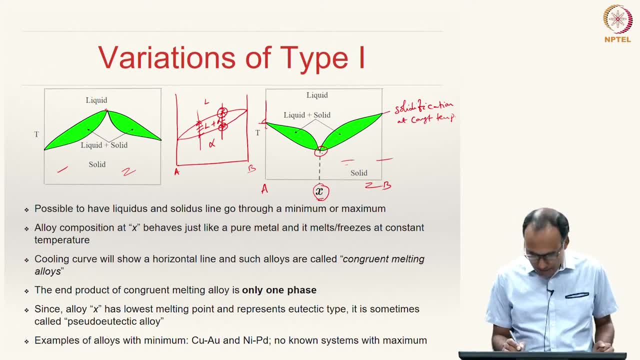 temperature. Now, if you look at this special case of an alloy with composition x, again, if you consider the solidification, the solidification is starting and ending at the same temperature. That means it is behaving like a pure metal in terms of its solidification. Solidification: 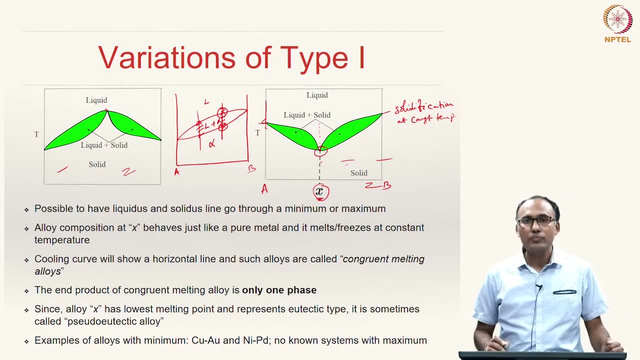 is happening at constant temperature and such alloys are called congruent melting alloys. That means the solidification happens for these materials at constant temperature and the composition of the alloy in the liquid state as well as in the solid state after the transformation will not change. So the end product of a congruent melting alloy is: 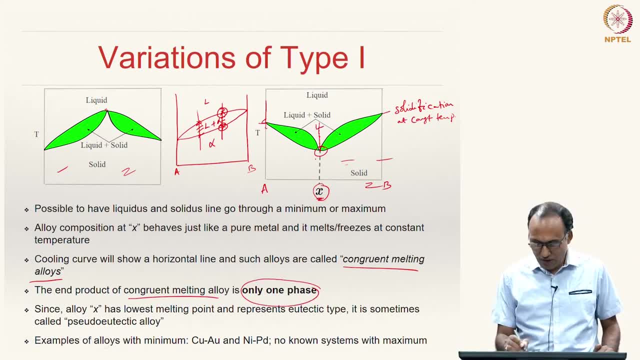 only a single phase alloy. So here you have liquid phase and it transformed to solid phase, right? So so is the case for your pure metals A and B. So the melting process or the solidification of pure metals is congruent in nature. Similarly, if you have any other alloy system, which happens- 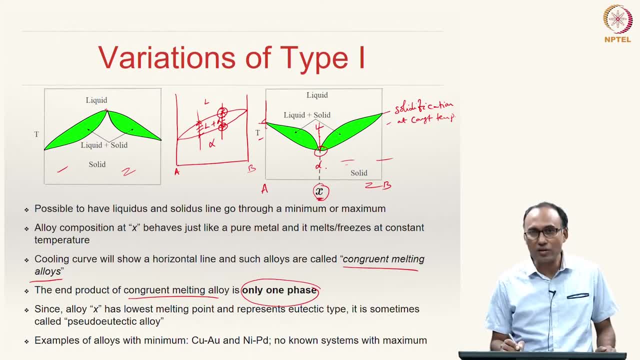 at constant temperature. but in addition to that, it does not only happen at constant temperature, but the end product it will be a single phase system. Here it is a single phase solid solution, alpha right. So since, for instance, if you see this, you 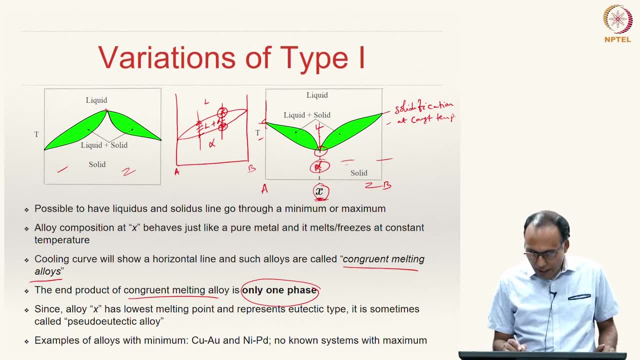 see this particular alloy composition X, the melting happens. So amongst all the alloy combinations between A and B, the alloy X has minimum melting temperature, right, minimum solidification or lowest melting temperature, And hence sometimes the. so this represents a special kind of a reaction, special kind of alloy types, called eutectic, but it is 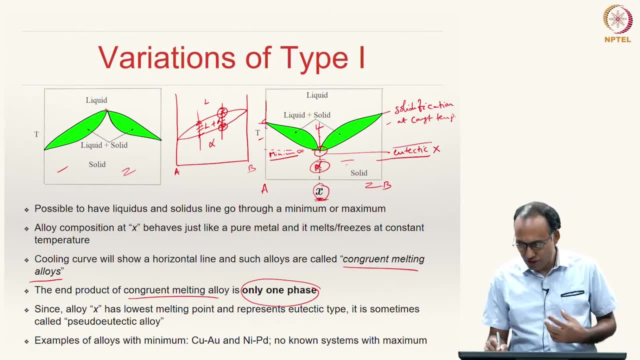 not eutectic, It is. it looks like eutectic, So it is not eutectic, It is, it looks like eutectic. We will discuss what is eutectic, but it looks like eutectic, but it is not. 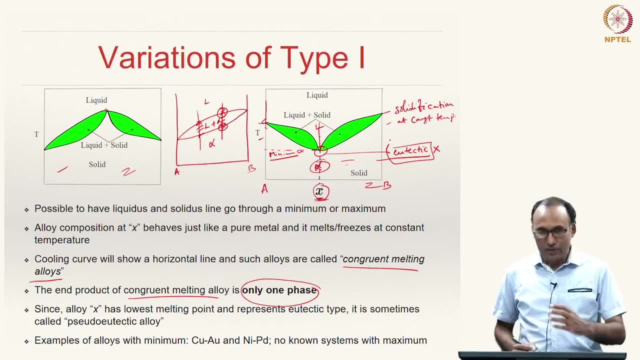 really eutectic. We will discuss the salient difference between a congruent melting phase and then eutectic phase. So since it sort of looks like a eutectic system, this is also called a pseudo eutectic alloy. It is not a eutectic, but looks like an eutectic alloy. 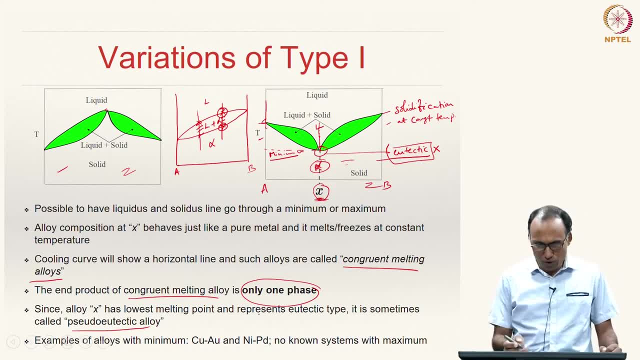 okay, You, the materials which show these kind of variations of type 1 isomorphous alloys with a minima or maxima at somewhere in between are not very common, but there are not- we do not know many materials which has a maxima, like we have shown on the left-hand side figure. 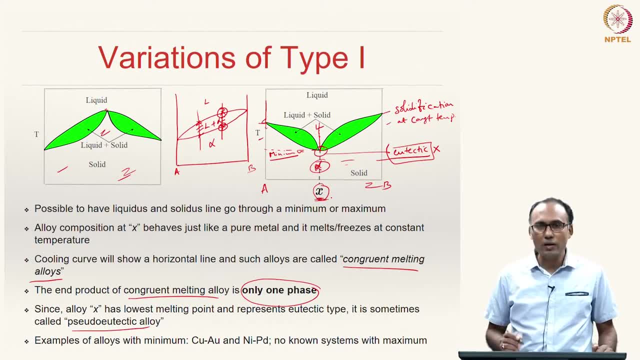 but there are evidence, evidences for alloy systems which show a minima like this, as it is shown in right-hand, right-hand side figure. The copper-aluminum, nickel-palladium systems are known to show this minima and there are. 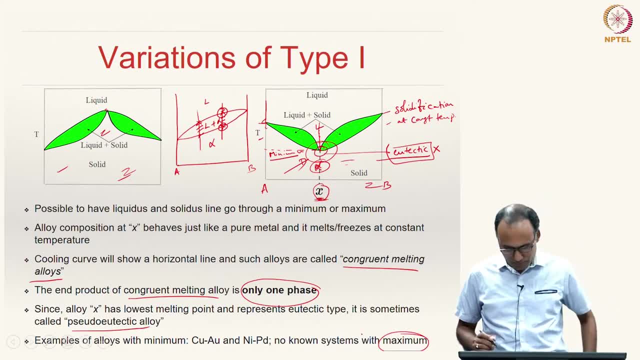 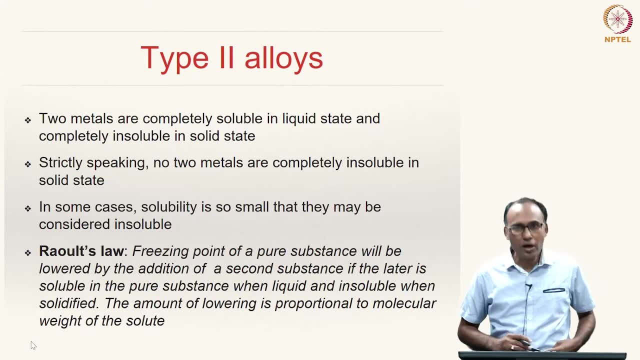 no known systems with maxima. okay, alright, So now, having discussed the type 1 alloys, now let us discuss the next type of alloys, called type 2 alloys. How did we define type 2 alloys? Type 2 alloys are characterized by the fact that they are completely soluble. 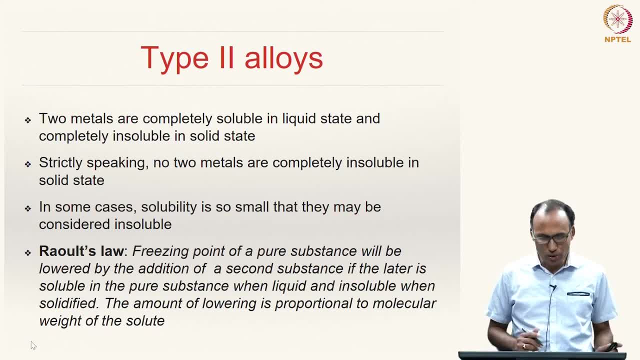 in liquid state but completely insoluble in solid state. So they are completely soluble in liquid state and completely insoluble in solid state. So that means what? When you are having in the liquid state, they are a nice liquid solution, but when you are solidifying, 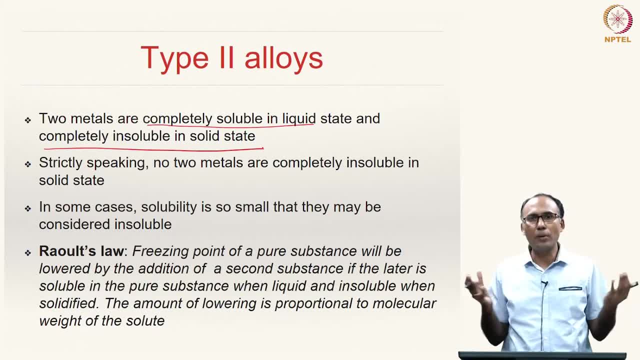 after solidification, they separate out into two different components. They will not make a solution. They segregate into A and B separately. That is what you mean by complete insolubility in solid state. This is a model system that we are choosing to study because, in reality, strictly speaking, no type of alloys are soluble in liquid state. So this is a model system that we are choosing to study because in reality, strictly speaking, no type of alloys are soluble in liquid state. So this is a model system that we are choosing to study. 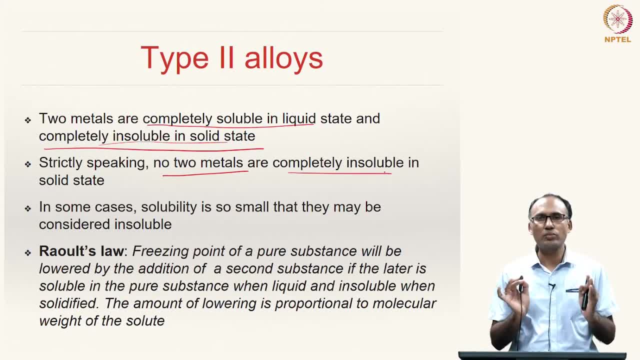 because in reality, strictly speaking, no type of alloys are soluble in liquid state, But two metals are completely insoluble in solid state. It is not possible to have complete insolubility. There will be very fractional, tiny amount of solubility may be there, but 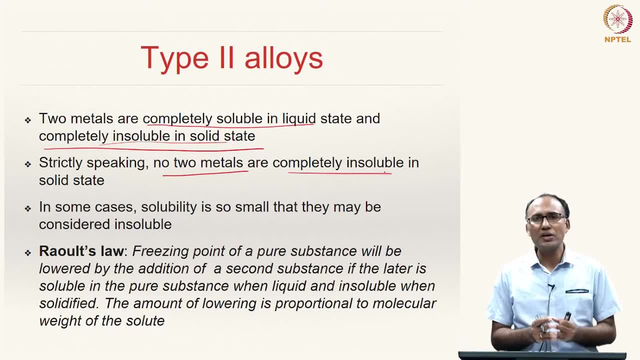 for all practical…. And hence, strictly speaking, we cannot say that there is complete insolubility in solid state. But if the solubility is very, very small, then you can sort of idealize that as complete insolubility in solid state. But even if there is a fractional, 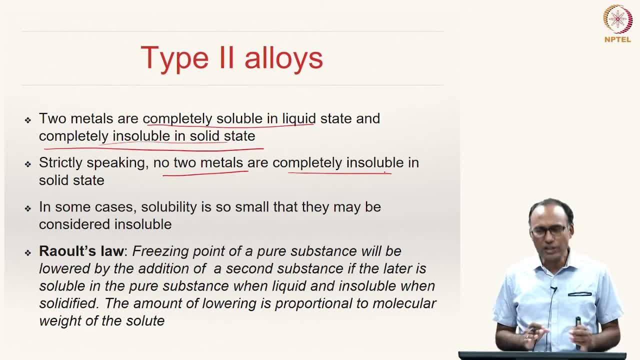 amount of solubility. you do not have to worry about that, due to the fact that we don't solubility. that will lead to certain differences that we will see at a later stage, but in this type of alloys type, whenever we are saying type 2 alloys, we have complete solubility. 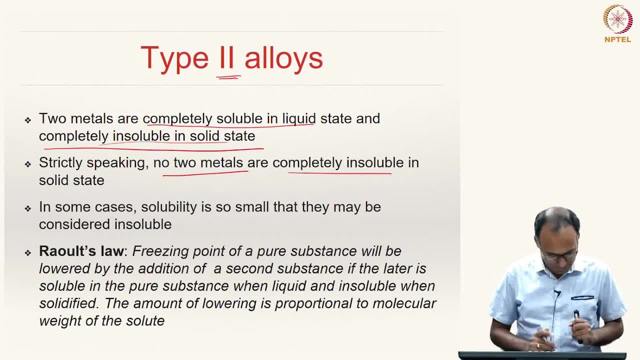 in liquid state and complete insolubility in solid state. So before we start looking at the phase diagram of this kind of type 2 alloys, we will first go through this Raoult's law, which states that the freezing point of a pure substance 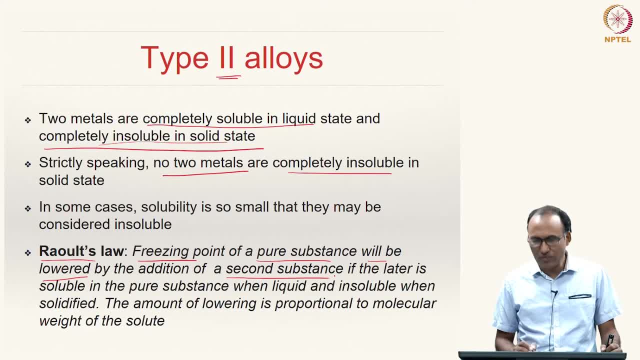 will be lowered by the addition of a second substance if the latter is soluble in pure substance when liquid and insoluble when solidified. That means if you have two materials, A and B, if they are, let us say you have A, and if you are adding A to B in the liquid state. 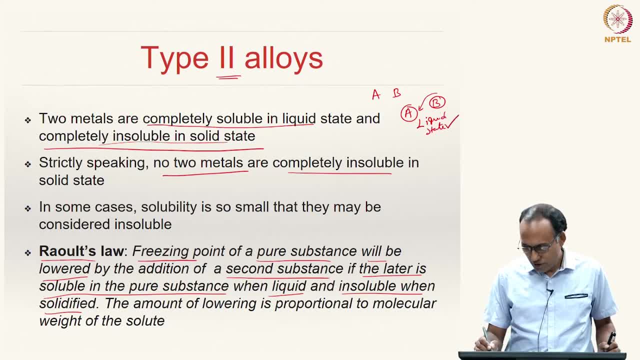 Okay, They are soluble, but A cannot join B in the solid state. If you have a system like that, then then Raoult's law says that the melting point of A will be lowered when you are adding B to that right the amount of lowering. how then? 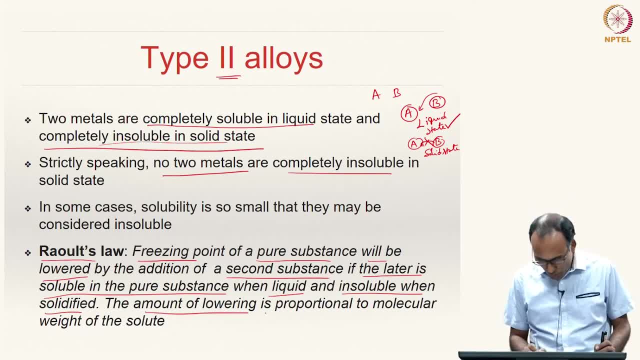 the melting point. how much? by how much amount it will be lowered? the amount of lowering is proportional to the Molecular weight of the solute. it depends on the molecular weight of the solute. okay, So the bottom line is that if you have two materials, A and B, which are completely soluble, 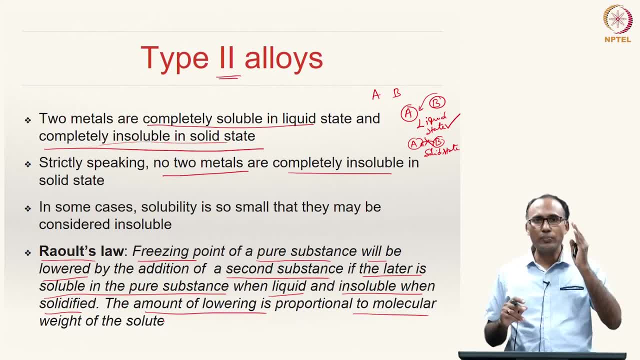 in liquid state and not soluble in solid state, then if you take pure substance A and if you add B, then the melting point of A will go down or the combination will go down in solid state, And if you take B and start adding A, then the melting point of B will also go down. okay. 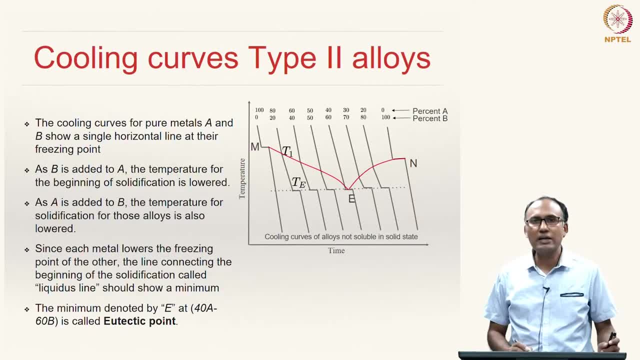 So that means, if you Let us say, for example, the A plant, Do you know that you can add B into the bottom of the solid state? us look at the cooling curves. So let us say: this is pure A, and pure A solidifies at. 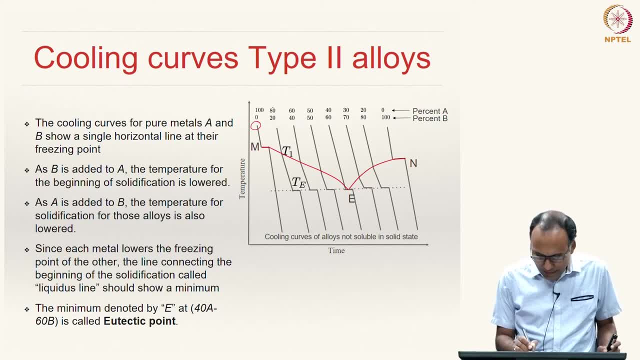 M, temperature M, and by adding So pure B solidifies at N. all right. and now when you are adding B to A, So that means it is 80 A, 20 B. according to Rawls law, the freezing point has to go down. So that is why the freezing point has gone down, but it will. 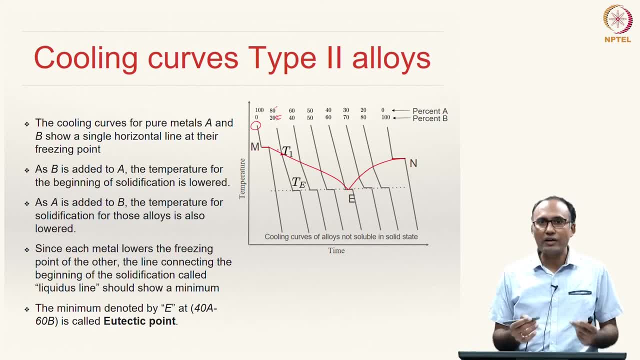 not solidify at constant temperature, because you will have- this is some liquid solution is there and hence it will solidify over a range of temperatures, right? However, if you so, that means the melting points of the alloys from left to right and the right to 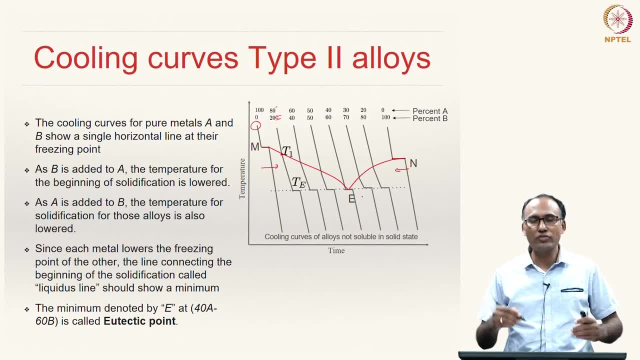 left are going to go down because of the addition of the solute atoms to the solvent cloud. So we see that there will be one particular alloy composition. let us say some, say in this case 40, 60. we have shown where, in again, the melting happens at constant temperature. It. 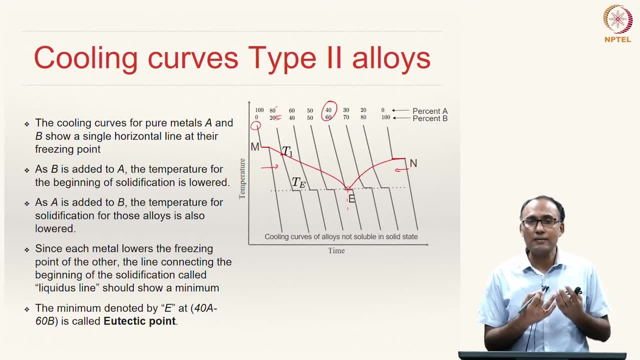 is like the congruent melting case, like it is like it solidifies. a melting or solidification happens at constant temperature, which means it behaves like a pure metal. So the cooling curve for pure metal A and B show a, This single horizontal line at their freezing point here, and as A, as B is added to A, the 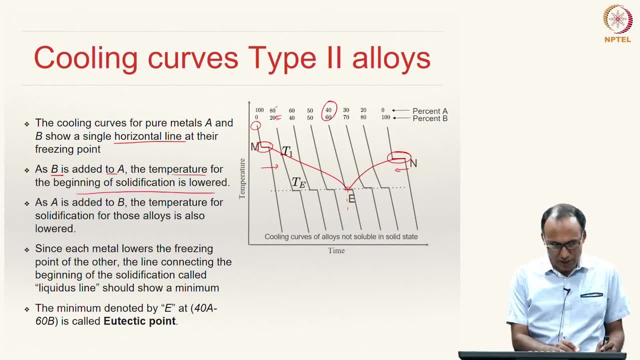 temperature for beginning of the solidification is lowered. Similarly, as A is added to B, the temperature for solidification is lowered for the alloys coming from the right, Since each metal lowers the freezing point of the other. the line connecting the beginning of the solidification line is called liquidus. should have a minimum somewhere here. So 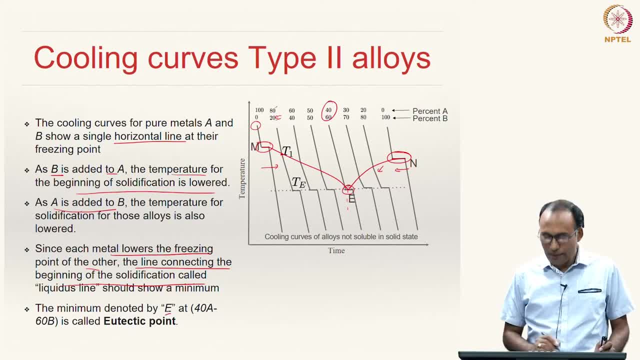 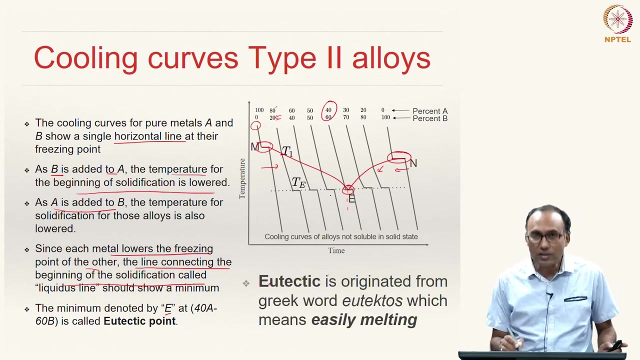 the minimum point point is what is denoted by E and that point is called eutectic point. That means, of all these combinations of alloys there is one particular combination, which at which the melting or solidification happens at the lowest temperature. okay, So the composition that 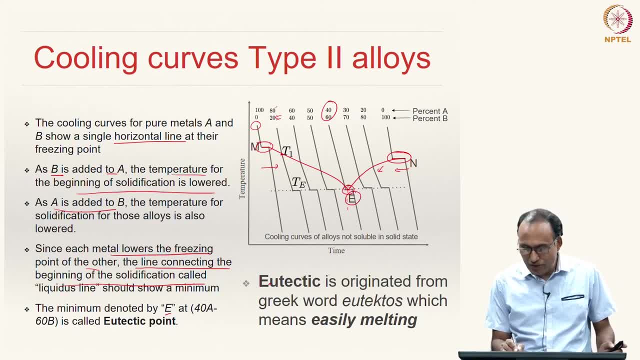 corresponds to that is called eutectic composition, and the temperature at which the solidification happens is a eutectic temperature. What do you mean by eutectic? Eutectic is a Greek word. It actually originated from a Greek word called eutectos, which means easily melting. 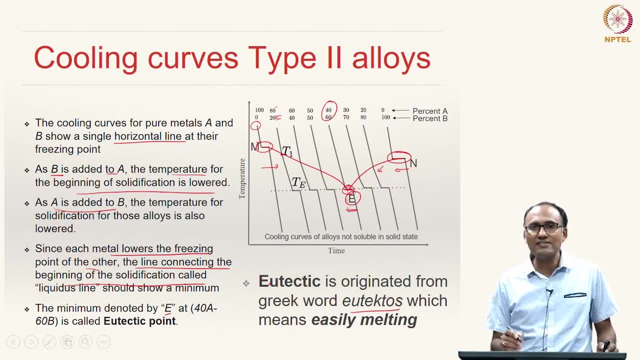 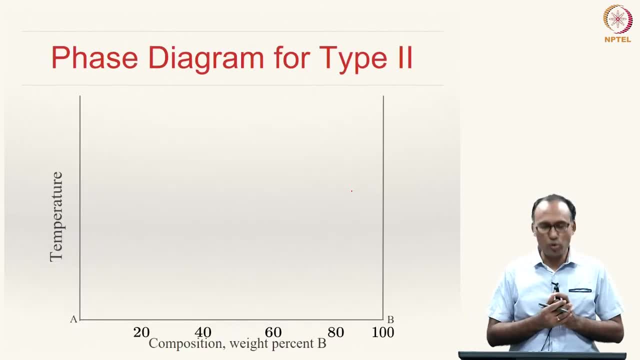 So, as you can clearly see here, this is the alloy that has the lowest melting point, and hence it is called a eutectic alloy. So this is something that we see in type 2 alloys. So let us look at the phase diagram from the cooling curves. Now let us look at the 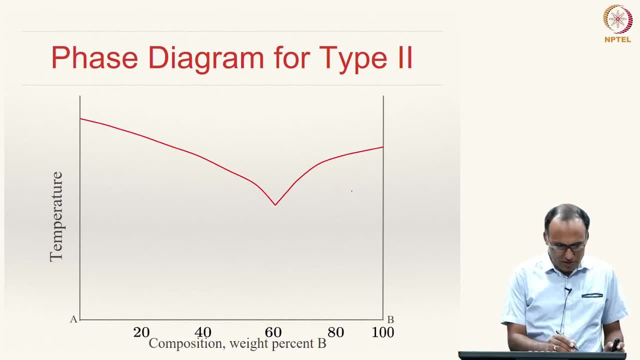 phase diagram, which is temperature composition. So that is our let us say. let us say: let us say the melting point of A and this is our melting point of B and, as we said, when we start, this is the solidification starting temperature. So, when you are, this is our. 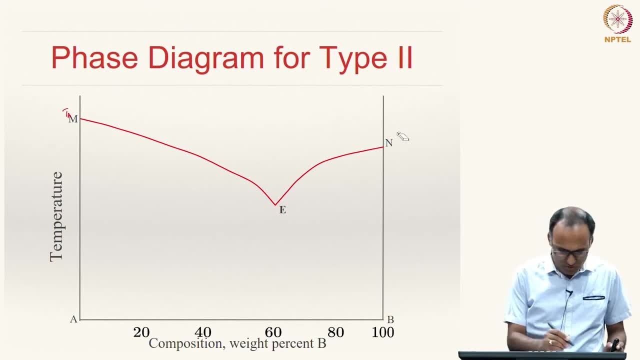 liquidus line, So M N. so here from the previous figure, M N I am choosing, and E is our eutectic point and that is our liquid solution, above that liquidus line and the melting point of A and melting point of B here, as is shown here, And then this green. 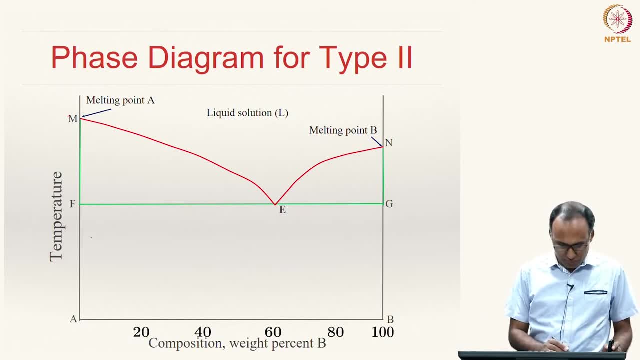 line that we have shown just now. that is So M, F, M, F, G, N is our solidus line. That means below that everything will be solid. above, above that you may have liquid plus solid. So in between the liquidus line, 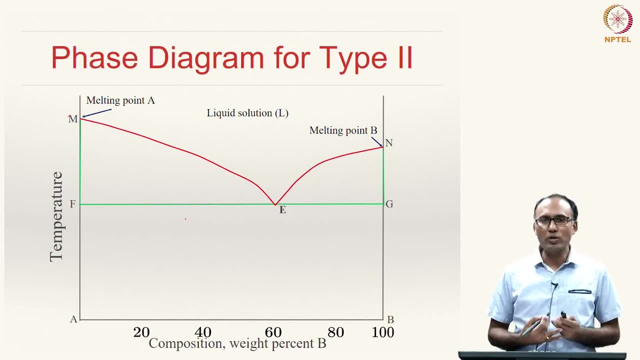 and solidus line you will have two phase region. Above the liquidus line you will have single phase liquid solution. Below the solidus line you will have again a solid phase and it may have two phases. but here we are only talking about a solid phase. So 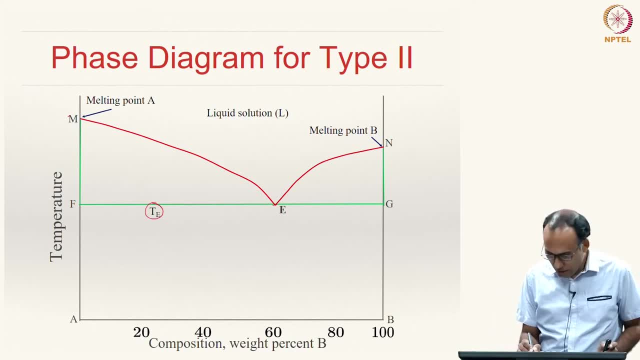 this temperature. So this temperature at which this eutectic alloy solidifies is called eutectic temperature, known as T E, and this is our liquidus line. and these green lines represent solidus lines, and here you have liquid solution, Since in the solid state the materials A and B cannot. 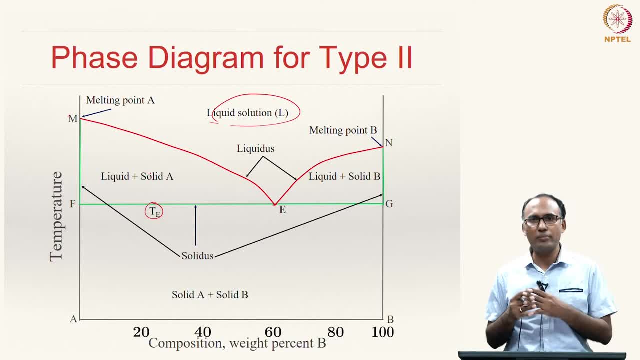 mix right. that is, they cannot. there is no solubility of A and B and B and A, and hence in the solid state they cannot be called solid solutions, because they cannot solidify each other in one another. So in the solid state we will not have solid solutions, but pure solids. So that is why. 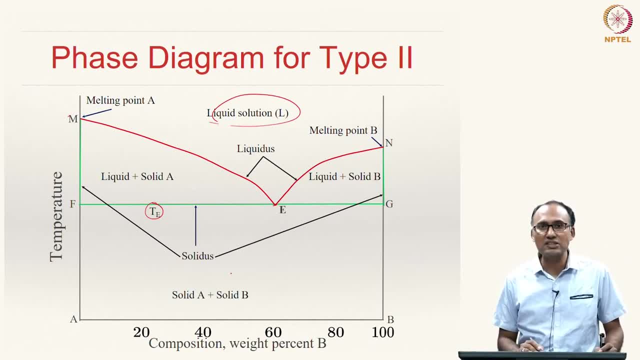 we are not representing the solid phases with Greek letters, but we are writing solid A and solid B. It is not a solid solution. It is pure solid A and pure solid B. So you will have two A and pure solid B. So the composition will be only even though it is a two phase region. 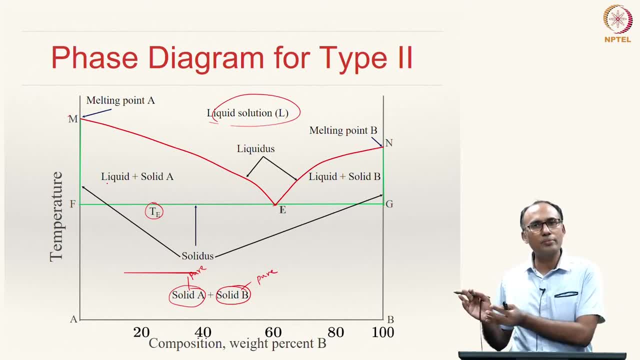 in some sense. So, but then 100 percent will be solid A, 100 percent will be solid B. their weight fractions are going to be different. that we will. we can get it through R tie line that we draw. And this is liquid plus solid A, because the here and here you will have 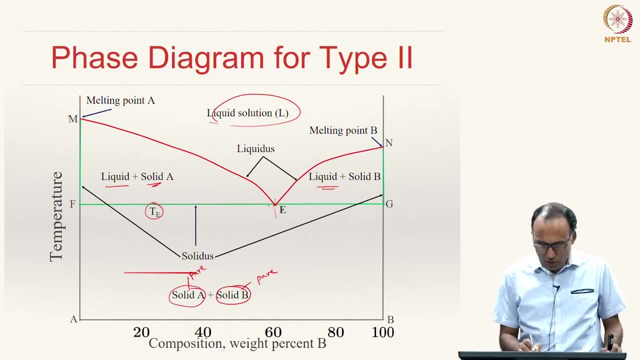 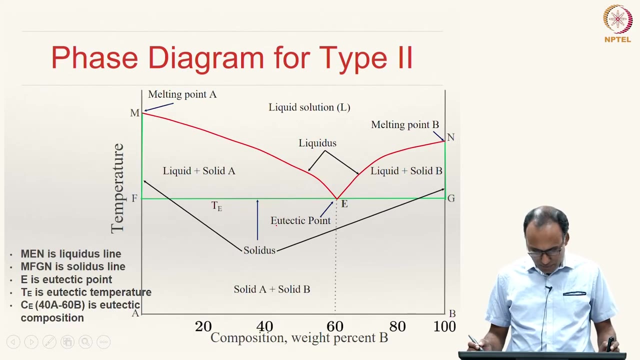 liquid plus solid B. So left to E you will have liquid plus solid A, because this side, you the solid, is solid A and right to that, liquid plus solid B, because this right side you have B And this is our eutectic point at 60 B. So, as we have already discussed, 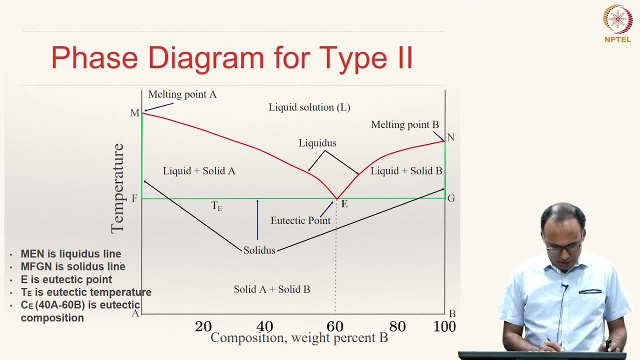 M, E, N is our liquidus line. M, F, G, N is our solidus line. E is our eutectic point to T. E is our eutectic temperature. C, E that I am calling. composition at E is what is our. 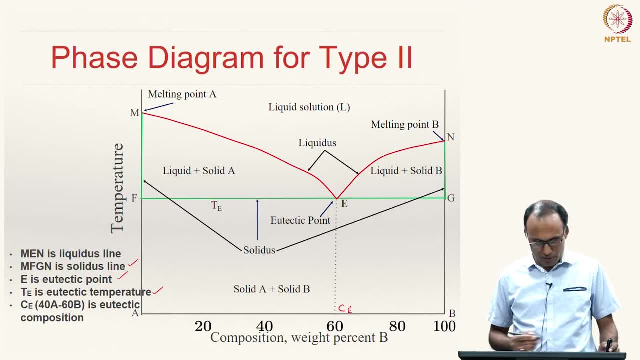 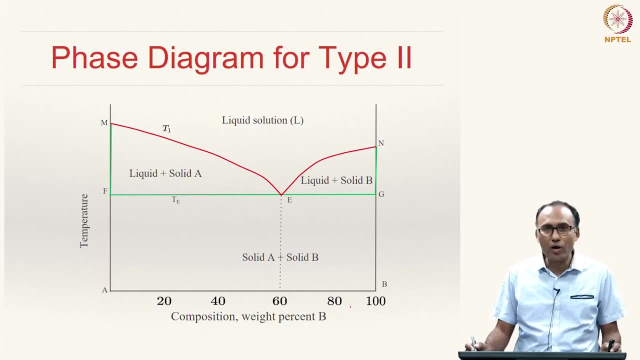 eutectic composition, which is 40 A and 60 B, Or we can simply say 60 B. So this is our phase diagram for type 2 alloys, and so this is our eutectic composition. So all the alloys left to this eutectic point are called hypo. 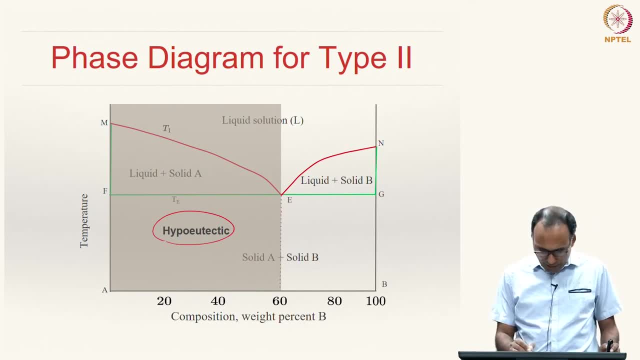 eutectic alloys. This particular alloy at composition C E is called eutectic alloy. all the alloy compositions left to that eutectic point are called hypo eutectic alloys. All the alloys compositions right to the eutectic point are called hyper eutectic alloys. That 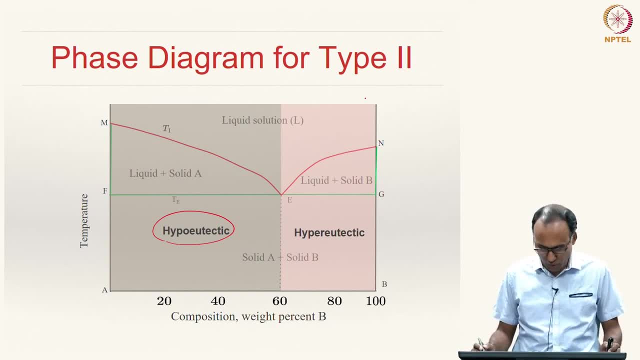 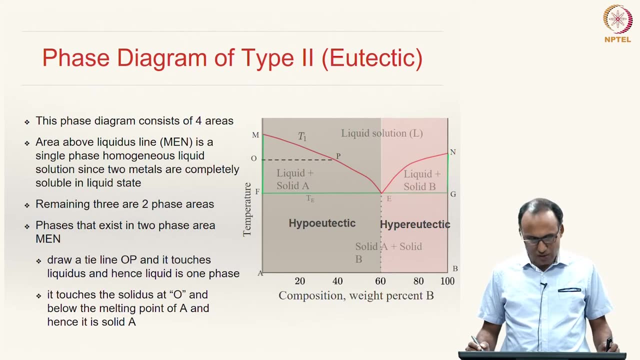 is a convention that we use in the rest of the module. So here we can clearly see that the phase diagram has four areas to be identified: The area above the liquidus, that is, above the liquidus line, M, E, N, M, E, N. this red line is: 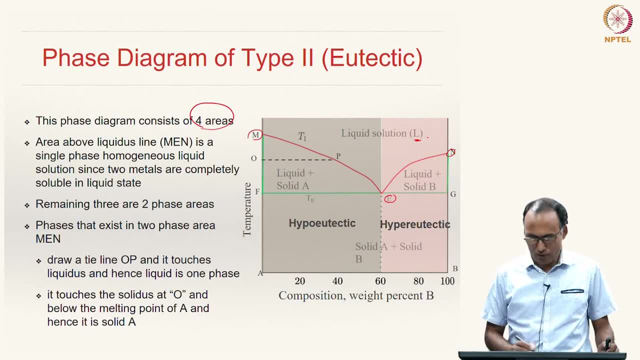 a single phase homogeneous liquid solution right L. So this is a single phase region which has, which is actually a liquid solution of two metals, A and B, which are soluble completely in liquid state, And there are the remaining three areas are two phase areas. This is liquid. 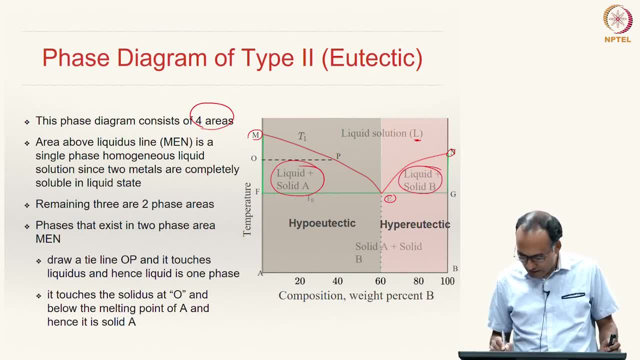 plus solid A is one area. liquid plus solid B is another area. solid A plus solid B is another area. right, This is a two phase region. So this should be solid B. this B is this B here is here. So this is a liquid plus solid. So solid A, solid A, this region, liquid. 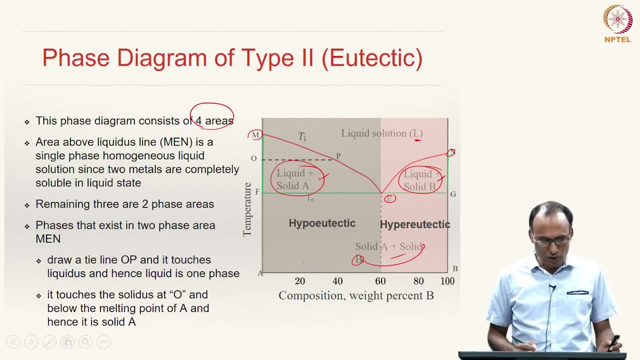 plus solid B, and here you have solid A plus solid B. All three are three two phase regions. ok, So in order to find the compositions, for instance if you want to find the phases that exist in two phase region, For instance, if you take this guy, you line draw, draw tie. 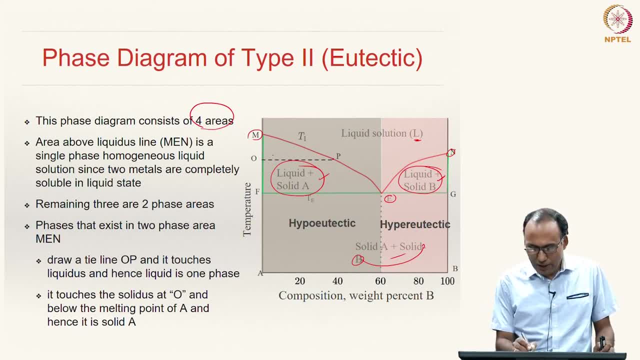 line O- P and it touches the liquidus line at P and the solidus line at O, which means the solid. In this guy, the solid composition will be solid A, 100 percent A, and liquid composition will be corresponding to this vertical. that is about 40, right? So now let us look at 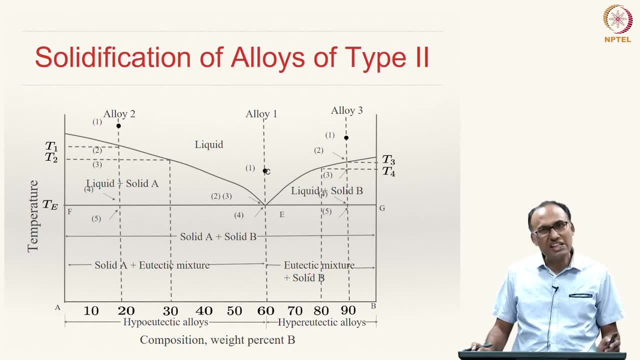 the microstructure evolution of three different alloys of type 2.. So type alloy 1 is having eutectic composition exactly, Alloy 2 is a hypo eutectic alloy and alloy 3 is a hyper eutectic alloy. and let us look. 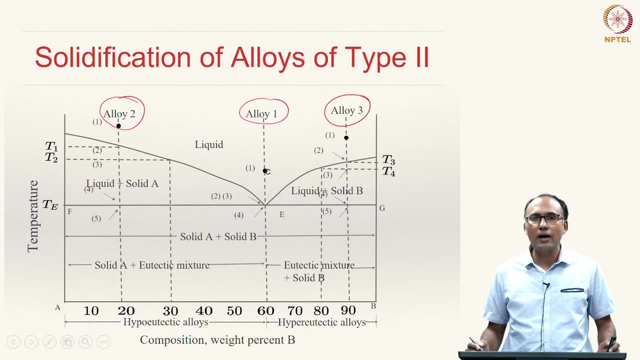 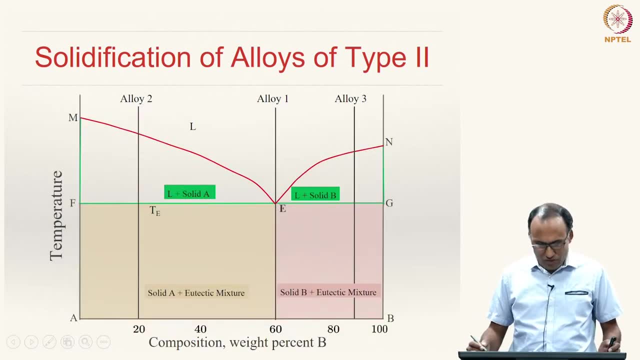 at how the microstructures look like for these three different kinds of alloys that we have discussed so far. alright, So, as we have already mentioned the above, the line M, E, N, solidus, liquidus line, you have all. everything is liquid, solution of A and B and you have three, two: 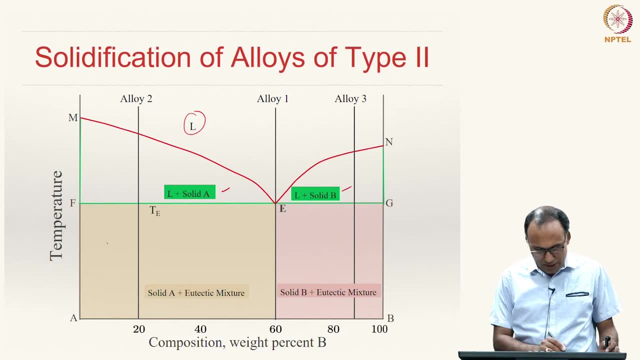 phase regions. So this is the hypo eutectic alloy. that is, hypo eutectic alloy will be a two phase mixture of solid A and a eutectic mixture. We we will see what do we mean by eutectic mixture. 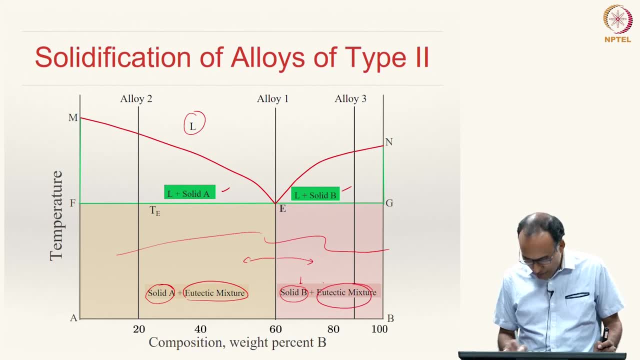 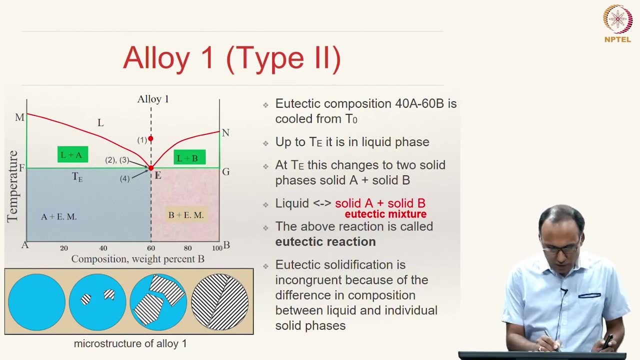 and to the right, you will have solid B and eutectic mixture. So, in order to understand this carefully, let us pay attention to each and every alloy. So now let us look at alloy 1, the microstructure evolution. So the alloy 1 is having a composition of 60 B on 40 A or 60 B, let us say which is cooled. 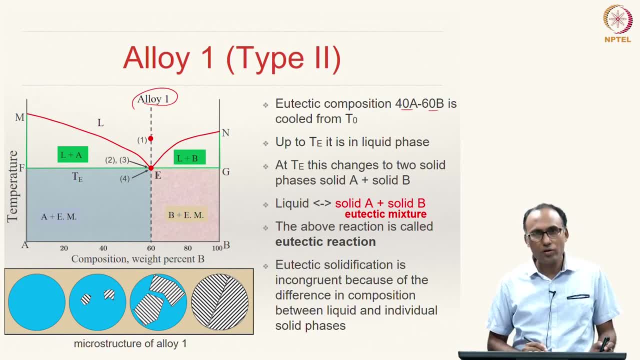 from the pressure at T 0, from, say, let us point one, So you are cooling down from 1. as you are cooling down, what happens? the liquids temperature, sensible temperature, sensible heat. it will be giving away sensible heat. as a result, the temperature of the liquid goes down Until it reaches temperature T E. that is your add. 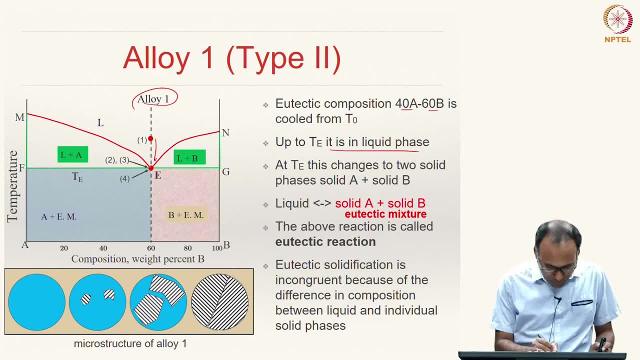 up to T E. in it is liquid phase at T E, at this eutectic temperature, what happens? So there is a reaction that is taking place. that is all. the liquid would transform to solid A and solid B, because above this it is liquid solution, below that it is again transforming. 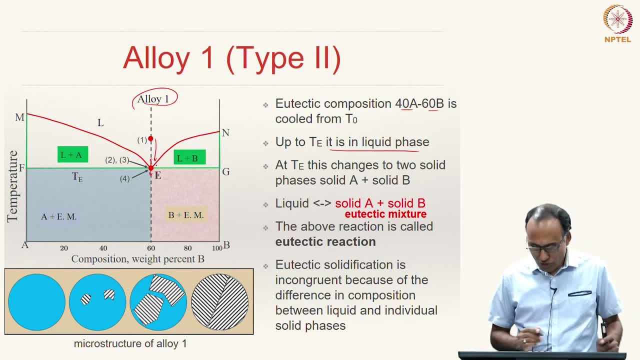 to two solids, solid A and solid B. So the liquid upon cooling at T e for this particular composition. So if you have a liquid solution whose composition is 60 B and when that composition is brought down to a temperature T e, that is this line, what 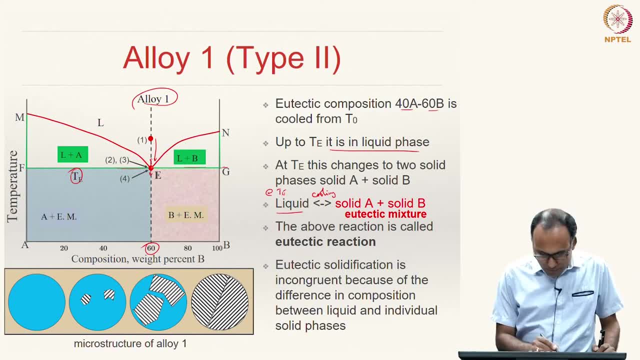 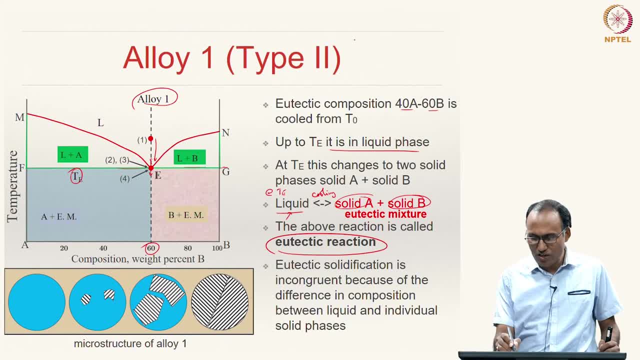 reaction is called eutectic reaction. So when we say eutectic reaction, what happens in a eutectic reaction? a liquid, upon cooling will transform to two solids, solid 1 plus solid 2. that is the definition of a eutectic reaction. And please note that this eutectic 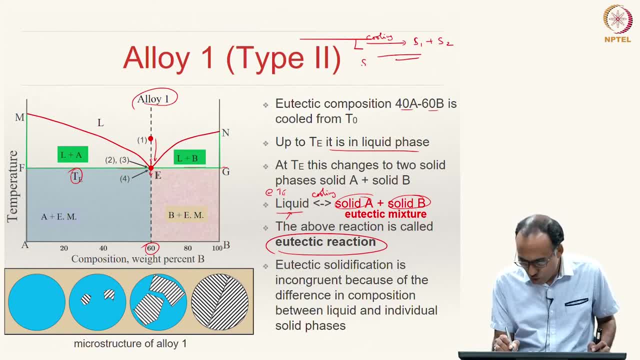 reaction is happening at constant temperature. that means this solidification happens at constant temperature, that is, T e. at that particular temperature the solidification happens. So whenever solidification happens at a constant temperature, we in the previous module when we said the pure metals solidify congruently, that means they solidify at constant temperature. 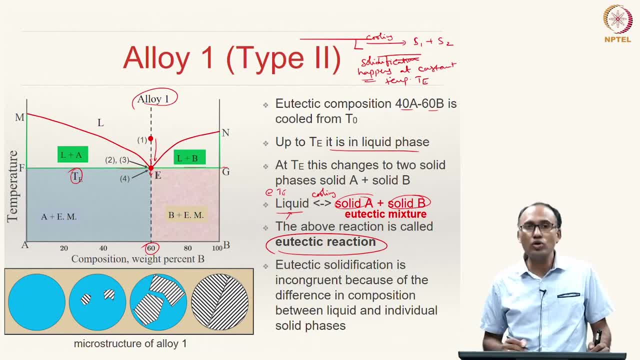 Now can we call this solidification also to be congruent? We cannot call eutectic solidification congruent. So it is incongruent because the difference, because of the difference in composition between liquid and individual solid phases, For instance, 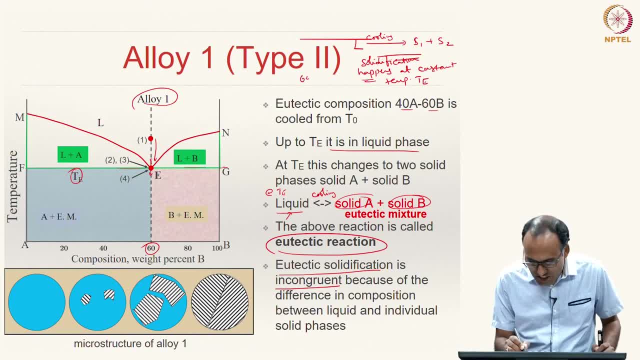 if you take the liquid solution has 60 B, 40 A. that is the composition of liquid solution. but when it is solidified, solid 1 has 100 A, solid 2 has 100 B, It has 20 B. So it has. 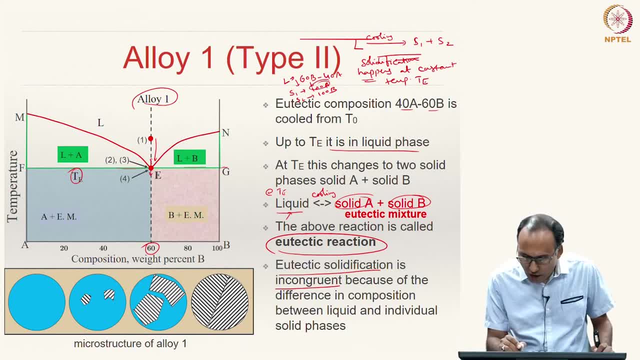 transformed from, it is solidified, but it did not retain the compositions. the compositions have changed right And hence, and it is not a single phase, it is two phase. in the congruent melting alloys, what happens? an alloy solidifies, but it will remain in one phase. but here, 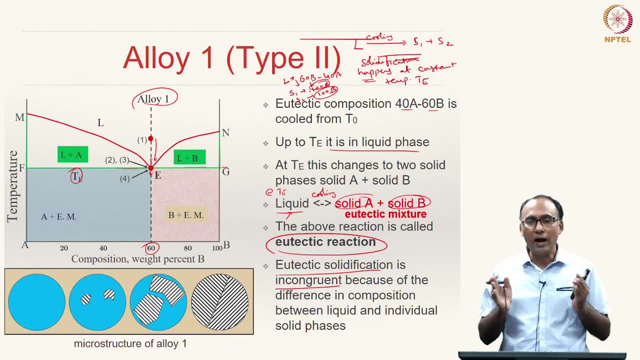 it is solidified into two phases and their compositions have completely changed, And hence a eutectic solidification, eutectic alloy, eutectic solidification cannot be termed as congruent, So it is in. it is incongruent in its nature. So now let us look at the microstructures. 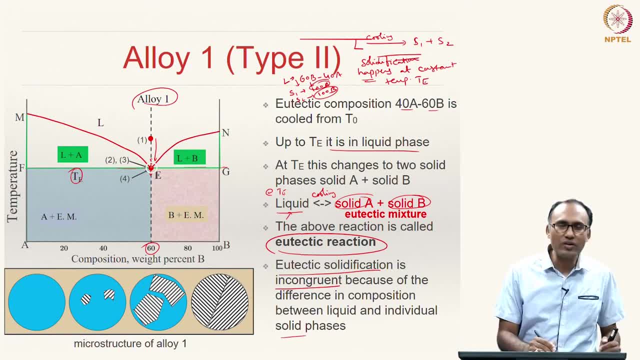 when you are cooling down, just at this point. So when now let us here, we are showing the microstructure as an evolution now in the time, at that point e, initially you have liquid and as you are cooling it down at that particular temperature, as you are waiting, your initial 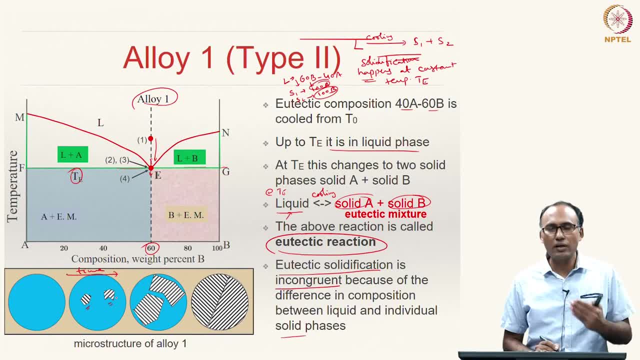 nuclei, of the solids nucleus starts forming And, as you are providing more and more time, the nucleus starts growing and complete solidification happens from liquid state to solid state. However, when it is solidifying what it does, when it is solidifying through eutectic reaction, it will form alternate layers of a and b. for 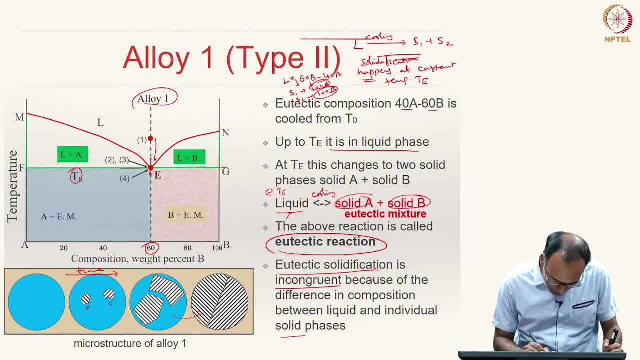 instance, in this picture you have the black. So here you have the black region and the white region. So let us say that the black region is a and the white region is b. That means the with the solidification. So now what would happen is that the solidification 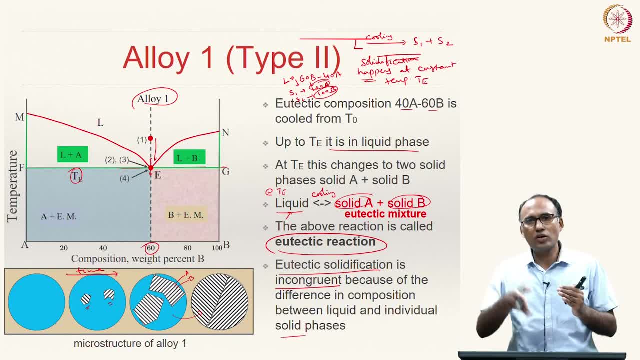 microstructure looks like alternate layers of solid A and solid B, So solid A and solid B. they will be forming alternatively, and such a mixture is called eutectic mixture. That is a typical nature of a eutectic, of a solid that is formed through eutectic reaction. 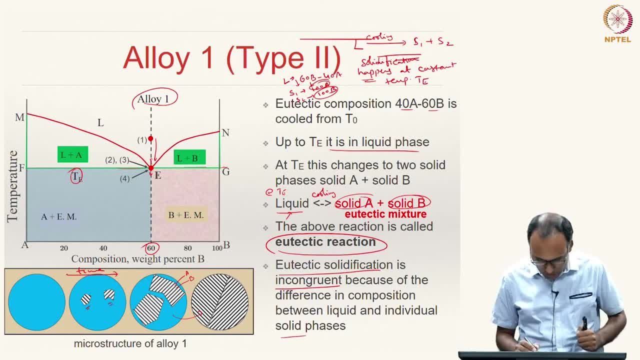 will have this alternate layer microstructure. So that is what is usually represented here, and please note that the microstructures that we are showing in these four graphs are only representative. They are in some sense they are schematics. They are not the real microstructures. 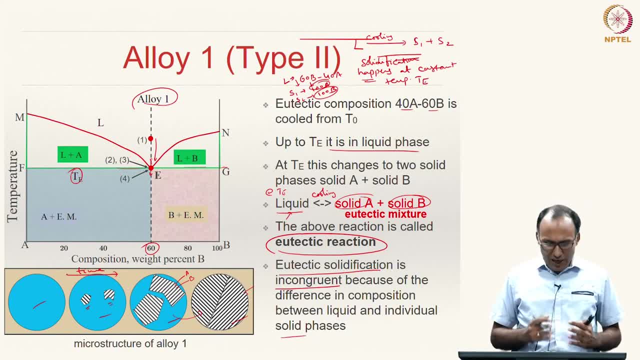 but then when you see the real microstructures under the microscope, you may have an alternate layer structure looking similar but not exactly like that. Also, the initial shape of the nuclei or grains can be very different. So here I have only shown two grains. It does. 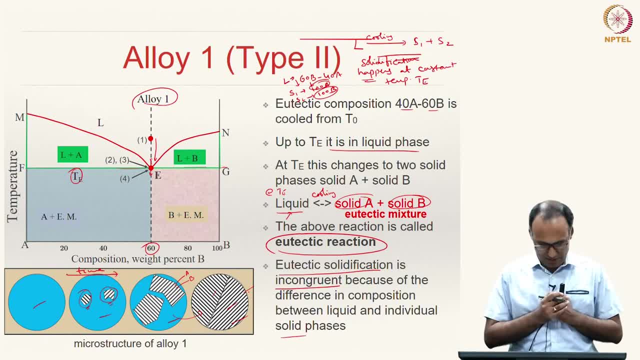 not mean that in reality also you will have two grains, You can have several grains. So the moral here… The summary of type 1 alloys… Sorry, in type 2 alloys, when you are looking at the solidification of alloy 1, which has a eutectic composition, it solidifies at a constant temperature called 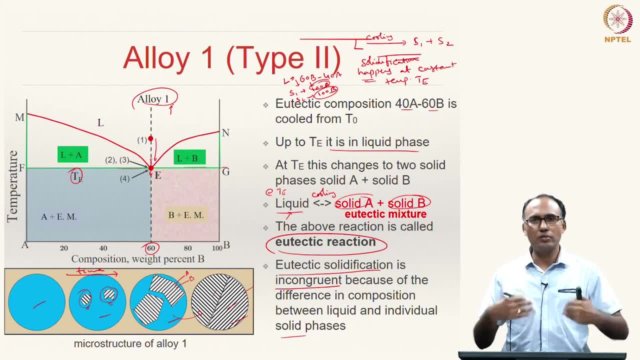 eutectic temperature and when it solidifies, it transforms into two solids, solid A and solid B, and the microstructures will be…. Microstructure will be alternate layers of solid 1 and solid 2.. Here solid A and solid B. 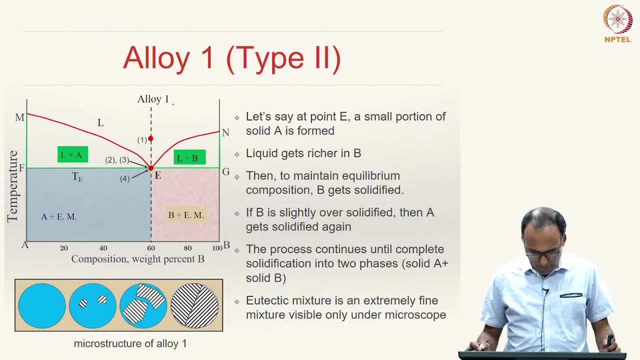 So let us see why, how this eutectic reaction is taking place. So let us say solidification is happening. So let us say, at point E from the liquid a small portion of solid A is formed. So let us say: you have the liquid solution, a small portion of…. Because in 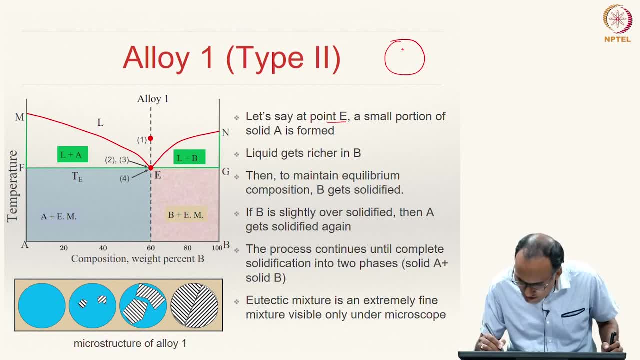 the solid state. they cannot be mixed. So this, let us say this: solid A is formed. So let us say: this is A. Then what happens? The surrounding liquid would become richer in B because some amount of A has gone away from that liquid. right? 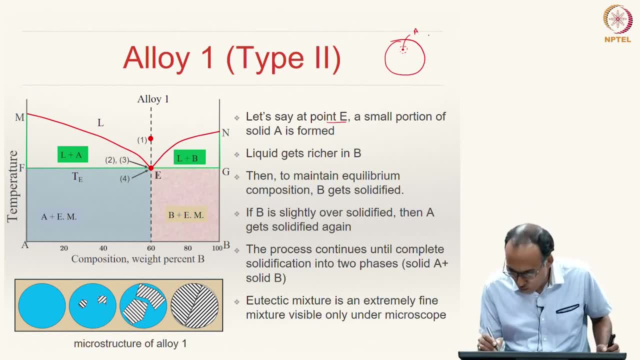 But the liquid's composition has to be…. So let us say now this is 60B, 40A, 60B. Now, let us say, a small amount of solid A has formed. So the liquid surrounding liquid, 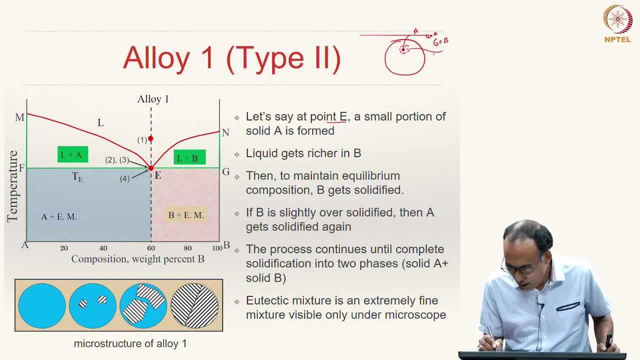 composition might have changed to 38 A, 72 B, sorry, 62 B. That means what happened everywhere else: it is still 60 B, but only the liquid that is surrounding the initial nucleus of A has become rich in B. That means this is not in equilibrium, because at that composition 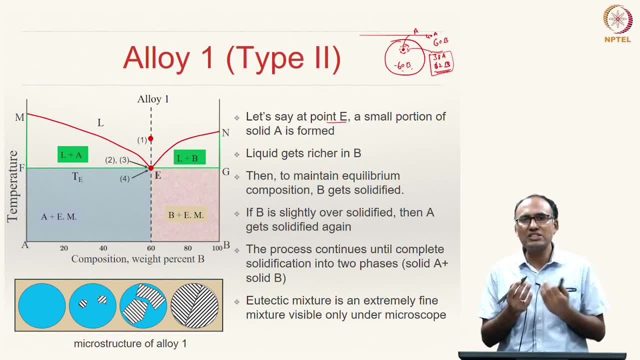 all the liquid should be. we have started with a composition of liquid which is having 62 B, 60 B. Now it has become 62 and hence, to maintain equilibrium, what it will do, it will give away this 2 whatever. So it will start to maintain equilibrium some amount. 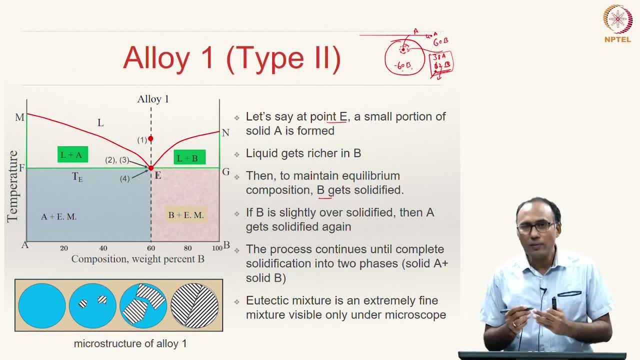 of B gets solidified. But it is possible that while the amount of B getting solidified, it may not actually exactly give away 2, it might give a little bit more. So if B is slightly over solidified, then what happens from that liquid? A gets solidified. 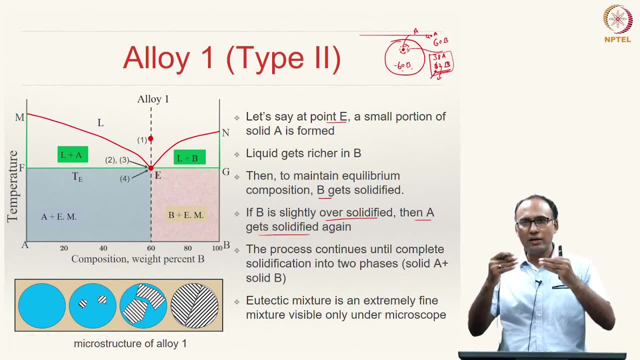 again. right like that, A and B try to solidify one after the other in order to maintain equilibrium. So the process is continued until complete solidification happens into 2 phases, that is, solid A and solid B, And under the microscope the eutectic mixture looks like an extremely 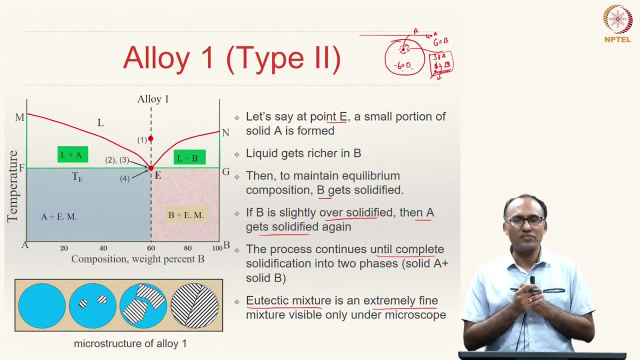 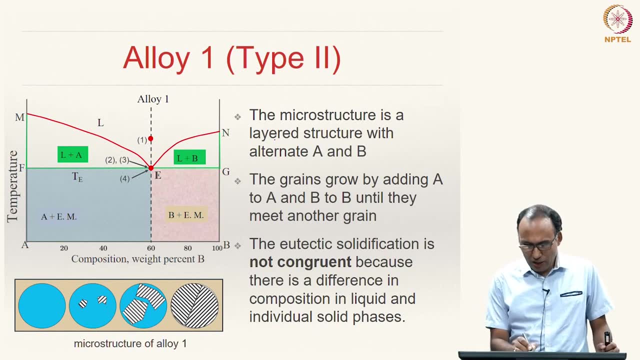 fine mixture of 2.. The eutectic mixture is roughly the same as the solidified mixture, until you know that the solidification of solid B gets better and the solidification of B gets worse vs omega 2.. So that means 1 over omega 2 is very, very good. however, you have to take into consideration 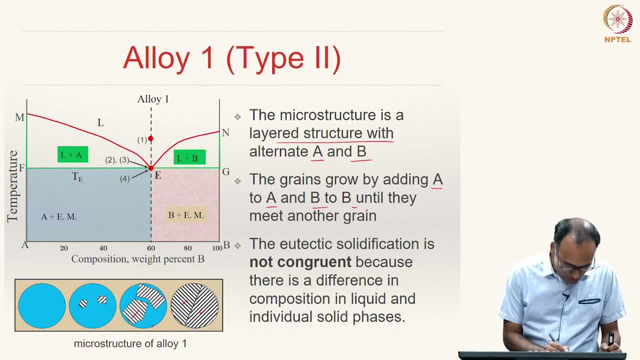 that in order to get the correct eutectic mixture. the eutectic mixture is very, very good. the eutectic mixture is capable of being absolutely fine. So, as I have already mentioned, the microstructure is a layered structure with alternate A and. 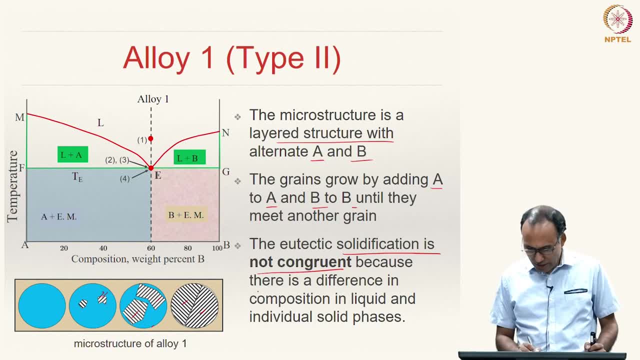 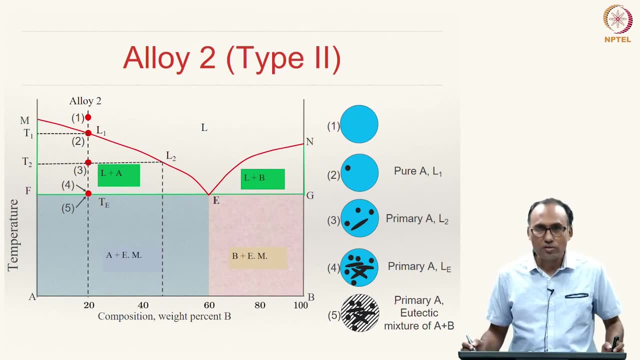 the eutectic solidification is not congruent because there is a difference in composition in liquid and individual solid phases. Alright, now let us look at the solidification of alloy 2 and its microstructure. So let us say that. so here 1,, 2,, 3,, 4, 5 states: 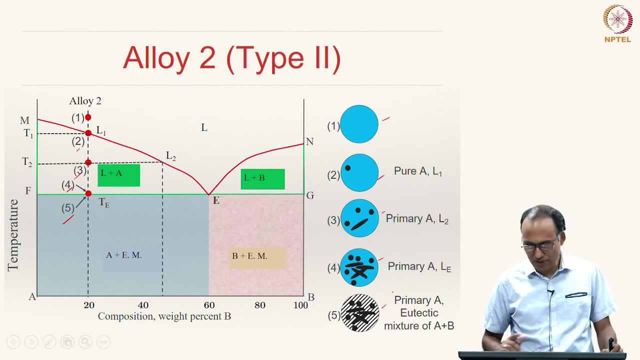 and the corresponding microstructures. here they again. they are schematics. please keep that in mind. whenever I am showing it is blue, that means it is liquid. So at 1, it is in liquid state. so this is liquid solution. and then, the moment you reach point 2, that 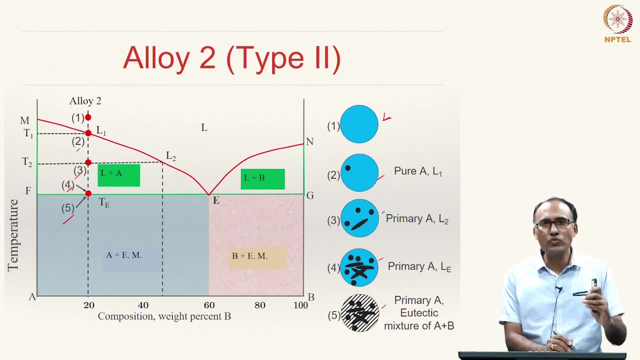 is on this liquidus line, you would be entering two phase region. That means a small, because you are now you are entering a two phase region. that means you draw a tie line. when you draw a tie line like this at temperature T: 1, right and this: 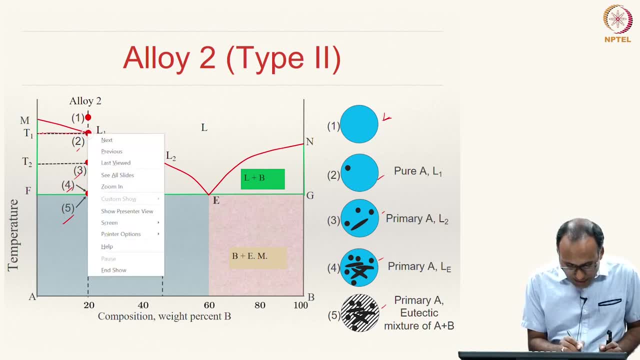 way I am calling L 1 state. then the tie line hits the solidus line. solidus line here, and that is what that represents: pure solid A, and that is the reason why you would form pure A And what will be the liquid, The liquid composition there, because its A is very small liquid composition. 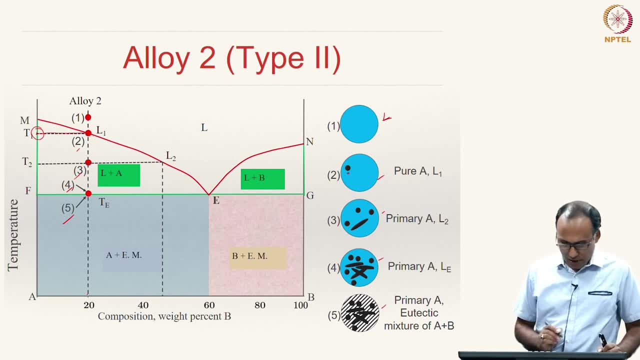 will be almost same: 20,, 20 B. and now let us say you are further cooling it down. and let us look at the state at point 3, at this position. So this is at temperature T 2, then you draw a tie line. the tie line hits the solidus line. 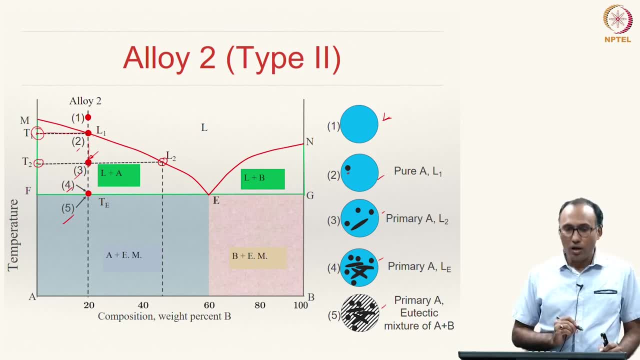 at this position and the liquidus line at L 2, that means the solid composition is again 100 A because it has hit at 100 A. So there is 100 A and what is the liquid composition? that is coming out to be something like 45 B. 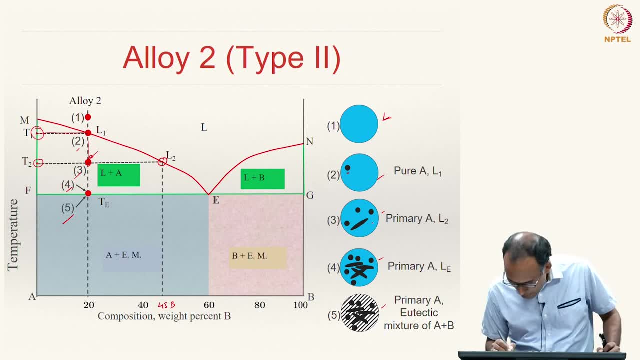 Right, Right, Right, Right, Right, Right. So here the liquid. initially, the liquid is 20 B. By the time it came here it has become 45 B. What happened? The liquid became richer in B because some amount of solid. 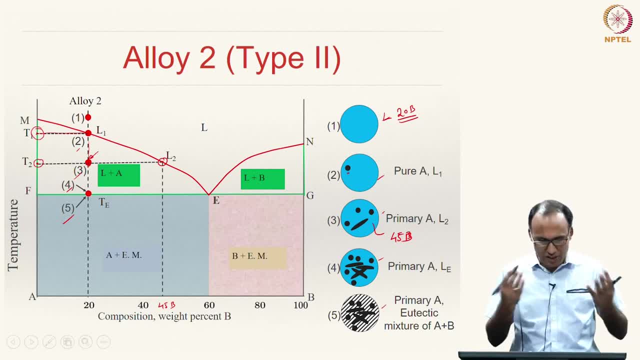 A is getting out of liquid and hence liquid starts becoming richer in B as you are coming down. That means, as you are cooling down, solid A is segregating out and the liquid is becoming a rich solution of B than what it has started off with. 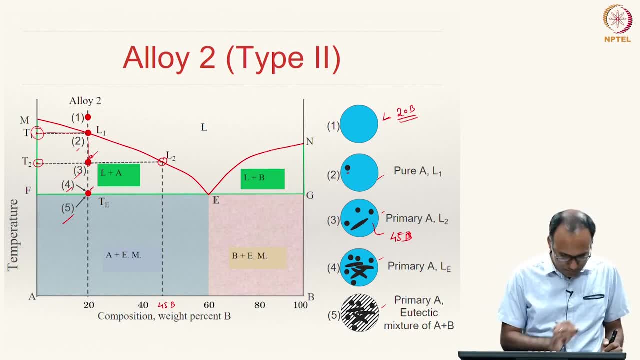 And now let us look at situation at point 4. here At point 4, what happens? You look at the, you draw a tie line that will be F. e will be my tie line in some sense. So the liquid, the solid composition, is 100. A fine, And now let us look at the liquid composition. 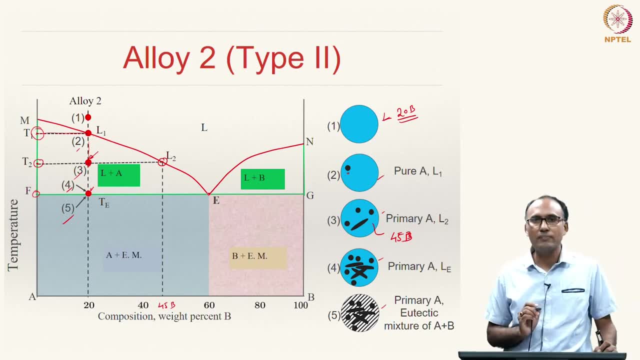 What is the liquid composition? Liquid composition is equal to eutectic composition. that means whatever liquid that is remaining here, the liquid that the remaining liquid has reached eutectic composition right 60 B. It has become 60 B. that means it has reached eutectic composition. And what is the temperature? 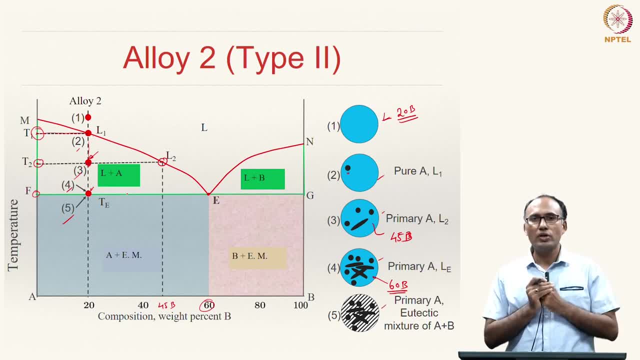 Eutectic temperature. Whenever you have a liquid solution at eutectic temperature and having a eutectic composition, what should happen? the liquid solution should undergo eutectic reaction. That means all the liquid solution should transform into two solids at constant temperature and that is what happens: All. 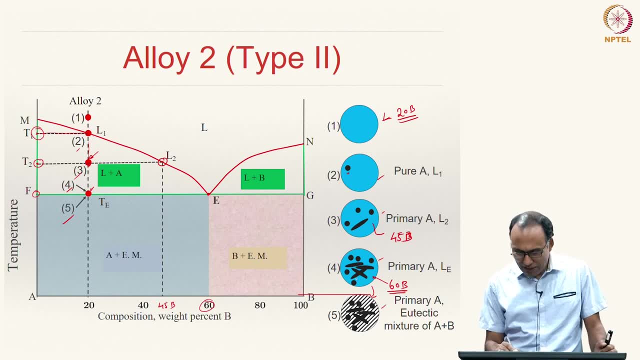 the remaining liquid solution. so you have some primary A that is formed until 0.4 and between 4 and 5 there is sufficient amount of time which we are not showing on the phase diagram, but remaining liquid solution would transform into eutectic mixture of A and B. 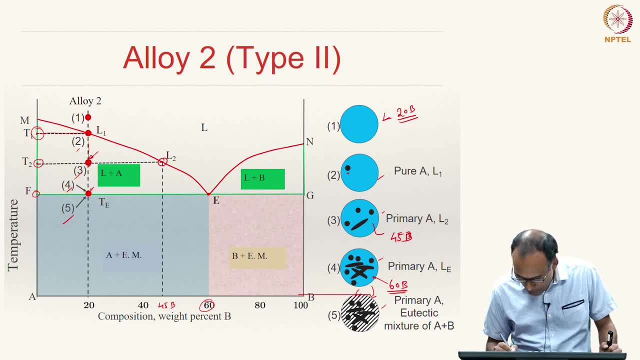 that is why you see alternate layers of A and B here: A, B, A, B and so on. So the microstructure, if you look at, you have some primary A and a eutectic mixture of A and B and that is the reason why here in this blue region hypo eutectic alloy, the microstructure is primary. 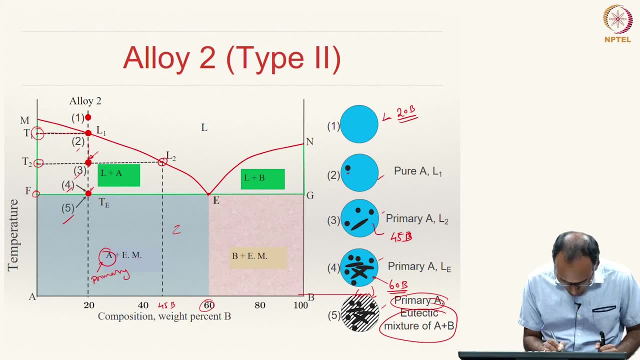 A and eutectic mixture of A and B. Please note that the eutectic mixture of A and B is also A. There is also some A in eutectic mixture and there is primary A where we. So, if you take, 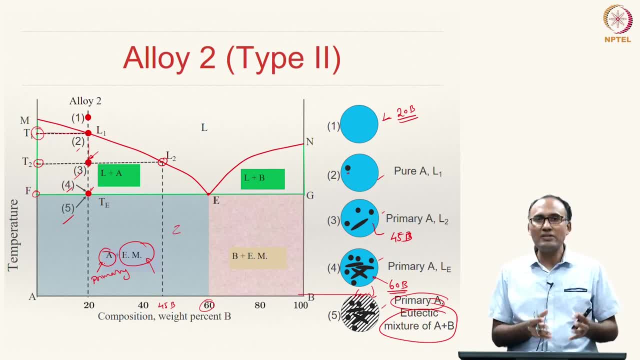 the total weight fraction of A that will be. there will be some amount of weight fraction that is formed through primary A and some amount will be in the form of eutectic mixture of A and B. So, as you again, another thing that I would like to point out: when we are 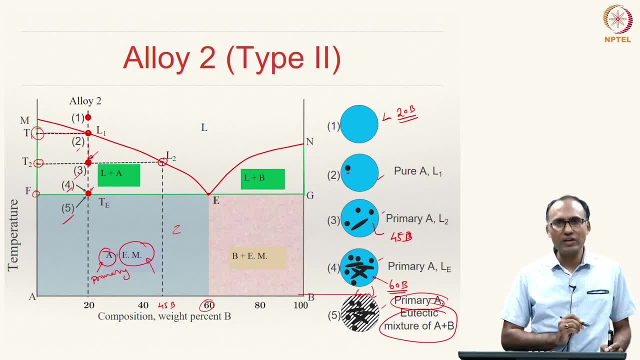 going from 0.2 to 0.3. what is the weight fraction of liquid? it is almost 100 percent is liquid. It will be very tiny amount of solid has formed. Now come to 0.3. what is the weight fraction? 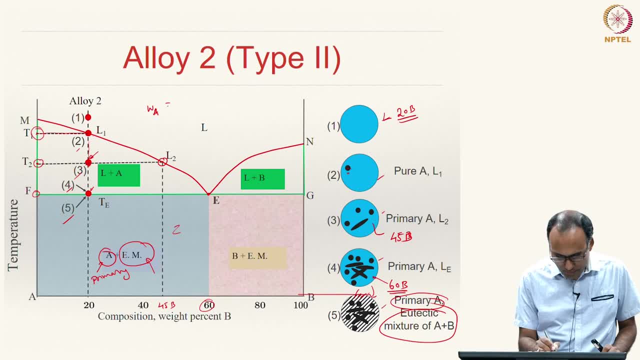 of solid or weight fraction of A. that will be so: t 2: 3 distance: t 2: 3 divided by t 2, l 2, what is t 2: 3? that is 20 divided by 45. right, this distance is 20 divided by 45.. That. 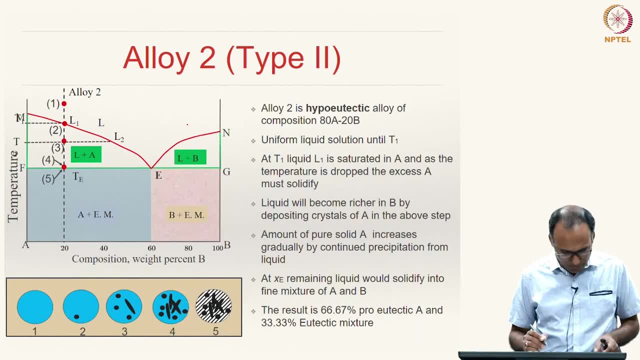 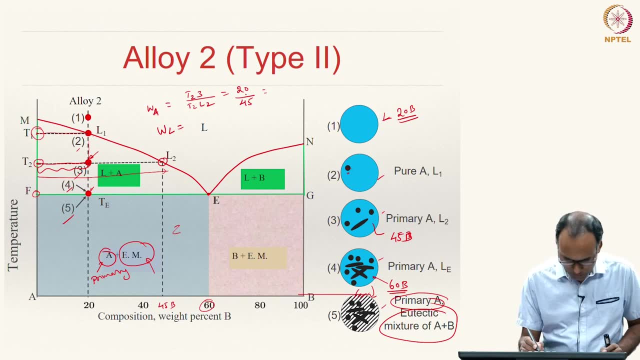 is the weight fraction of A and weight fraction of the remaining liquid will be… I am sorry. I am sorry, The weight fraction of A will be this distance, because the portion that is touching the liquid as line is what we need to take. So that is 45 minus 20, because this distance will. 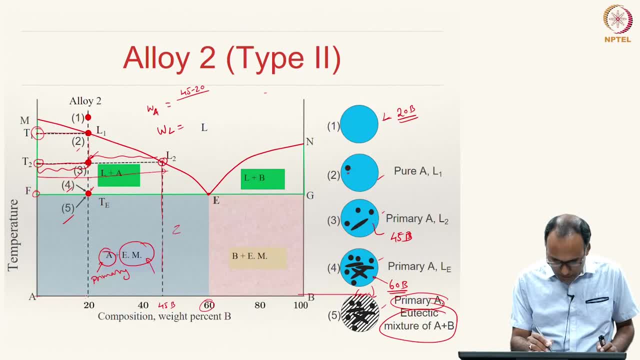 be total distance minus this distance, 45 minus 20 divided by 45, and this is weight fraction of liquid, is 20 by 45, that is 15 by 45, now 25 by 45, and this is 20 by 45.. 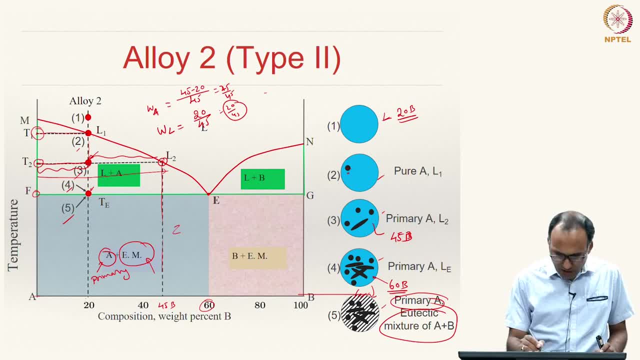 So the weight fraction of the liquid has come down and the weight fraction of solid has increased compared to 0.2 and by the time you come to 0.4,. what is the weight fraction of the liquid at 4?? Weight fraction of liquid at 4 will be 20 by 45.. 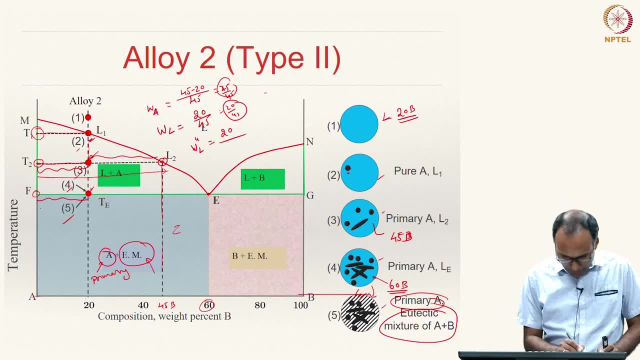 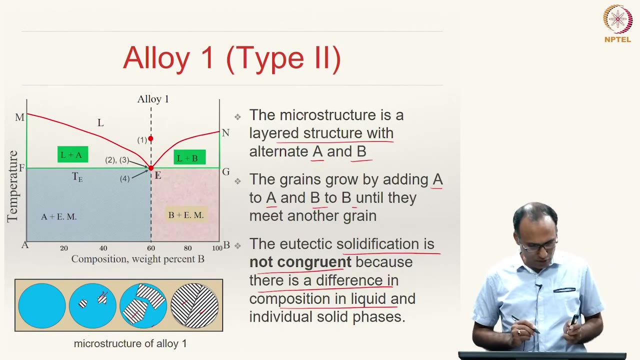 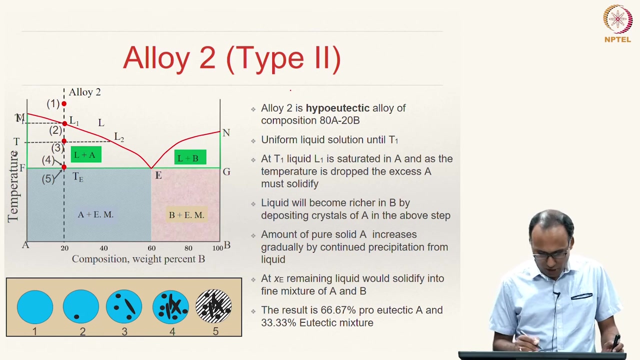 because this distance is 20 divided by 60, that is one-third, that is 33.33 percent. So let us carefully look at it now. So, alloy 2, let us go through it once again: Alloy. 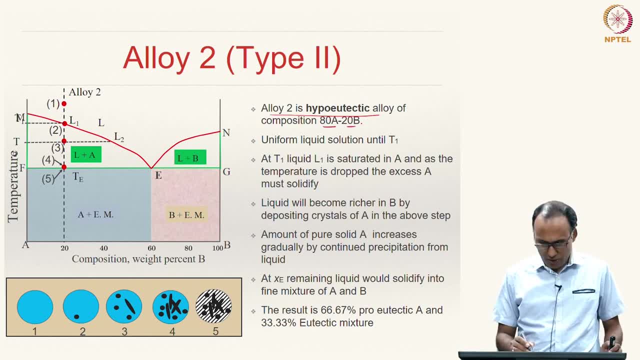 2 is hypo-eutectic alloy of composition 80 A and 20 B until temperature T 1, that is this guy. uniform liquid solution until T 1.. At T 1, liquid L 1 is saturated in A As. 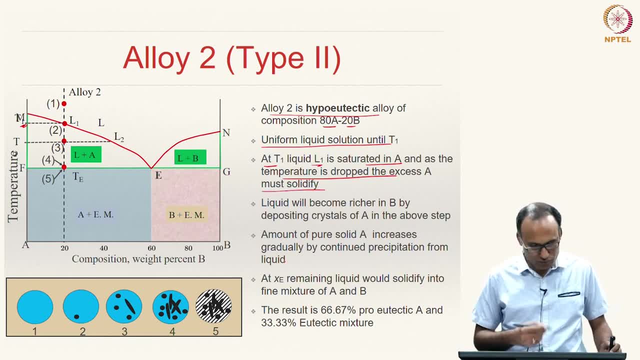 the temperature is dropped, the excess A must solidify. So as you are coming down, the excess A must solidify, And as we are coming down, the liquid becomes richer in B by depositing crystals of A in the above step. So as we are coming down, you will have a. 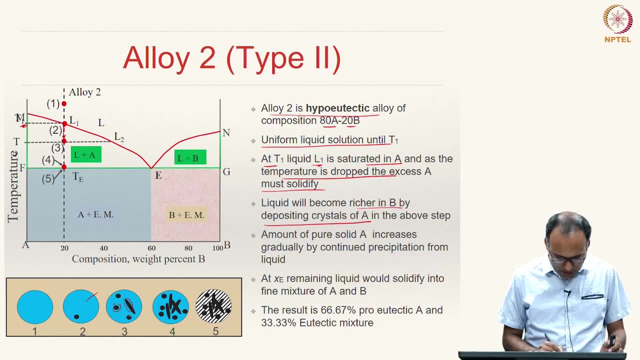 liquid becomes richer in B and you get out the crystals of A, solidifying out alright. And as you are going from 1 to 4, the amount of pure solid A increases gradually by continued precipitation of solid A from liquid. At x- e, that means at this position remaining. 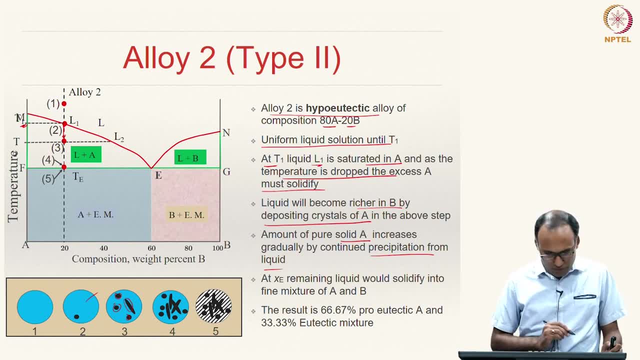 liquid. So what happens is, by the time you reach here, So the remaining liquid will would have reached the eutectic composition and that would go through a eutectic reaction and then solidify into mixture of A and B. And we have seen. 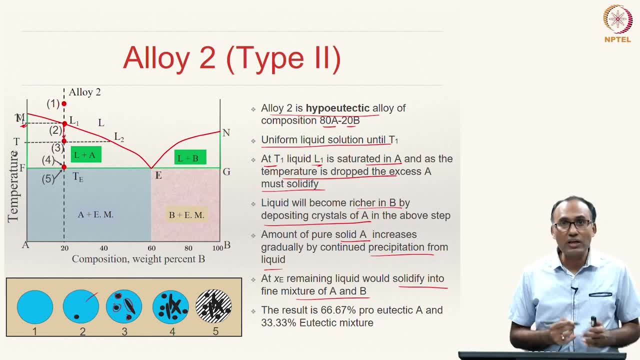 that the what is the weight fraction of the liquid? just above this point, The weight fraction of liquid liquid, weight fraction we have just now calculated, that is equal to 20 divided by 60, that is 33.33 percent. So this 33.33 percent we have just now calculated. So 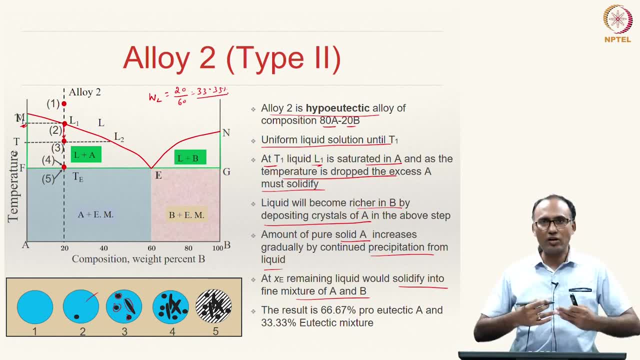 this is evidence that you have added that solid B, this process, in a mixture of A in 1 to 3.. So for eutectic process, we are still having lived up this point here. if you have stress kilos or higher concentration, so we are still having a concentration in that position. This is the proof of EUTECTIC哱 Kasimnyi using INP principle. So, like we have seen, with solid B there would be slight variation in our那麼 we will go, given thisi be for solid B. for solid B, go with EUTECTIC哱 Kasimnyi using INP principle. 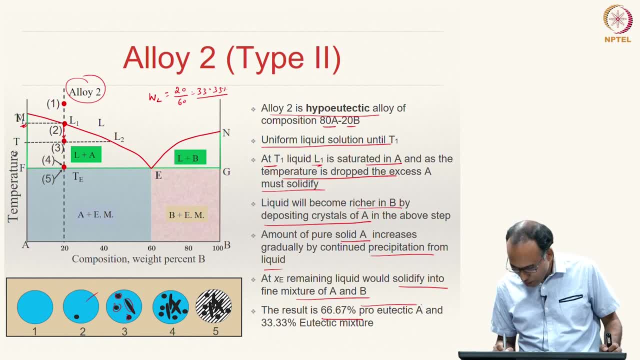 So, if it is very possible, that you would check the equation Amp, Theta for all these A, which is also known as pro eutectic A, The primary A also has another name, pro eutectic A. That means this A has formed before the eutectic reaction has taken place, That is. 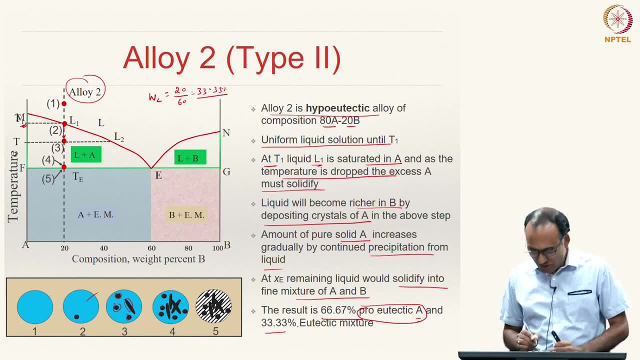 why it is called pro eutectic A, And the remaining 33.33 percent will form eutectic mixture. due to the eutectic reaction of the remaining liquid, which is 33.33 percent in weight, And that transforms to solid A, alternate layers of solid A and solid B That we are 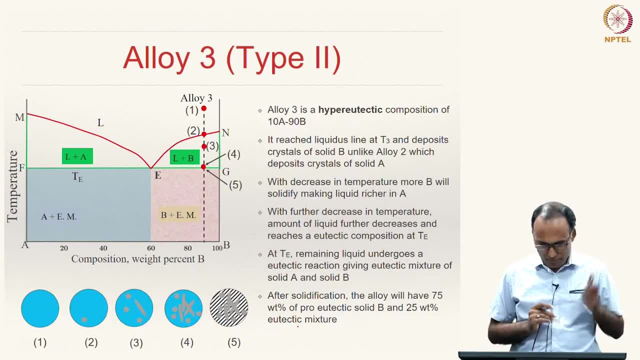 calling as eutectic mixture. And now let us look at alloy 3,, which is exactly similar, except that if you draw a tie line at point 3, this tie line hits the solid solidus at pure solid A, That means the solid phase. 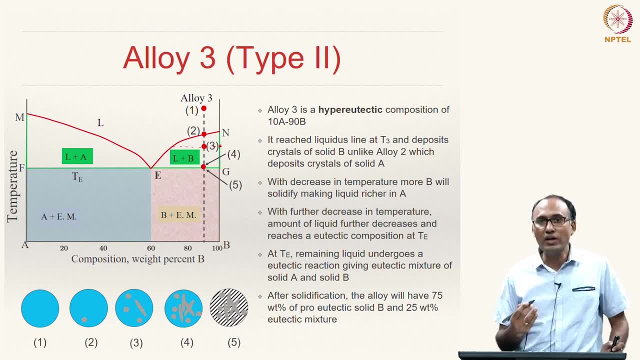 should be pure solid B And hence the solid phase that is precipitating from the liquid should be pure B. That is why it is pure B. Now you understand why we have written liquid plus solid B. We have written liquid plus solid A here because when you draw a tie line in this region, it 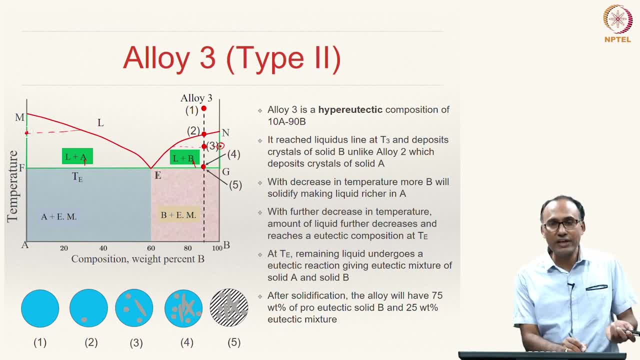 will hit the solidus line at pure solid A And hence it has to form pure solid A. Here it will hit the pure solid B line And hence it has to form pure solid B. So all the alloys here will have pro eutectic B. That means this gray line, gray one is what we call pro. 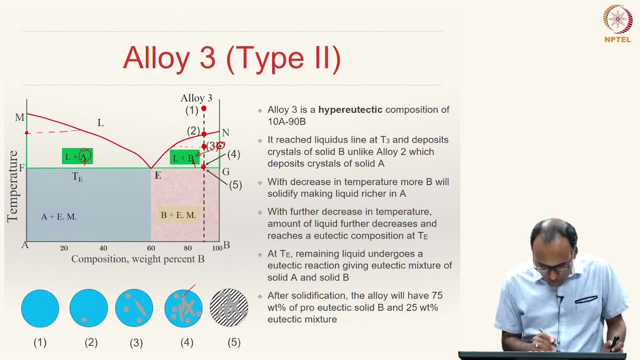 eutectic B. And by the time you reach at point G again your liquid solution will have the composition of eutectic solution. eutectic composition Again. the remaining liquid solution will transform to eutectic mixture of A and B. 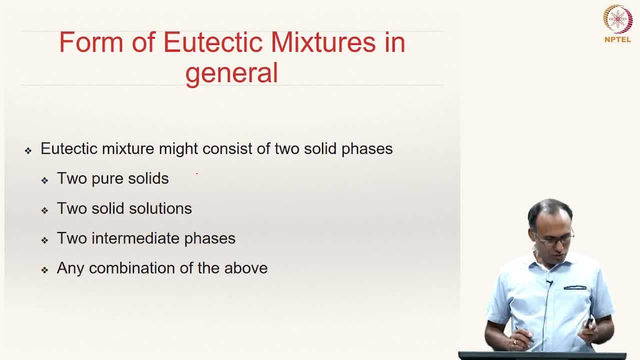 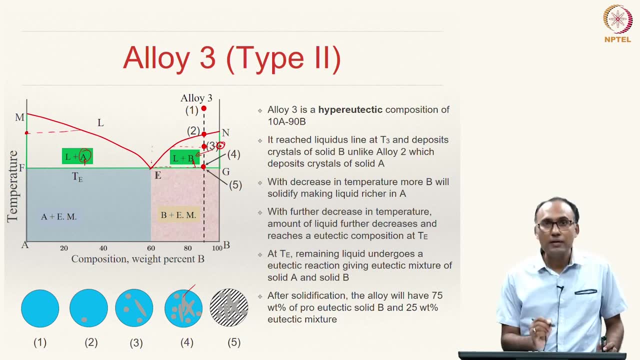 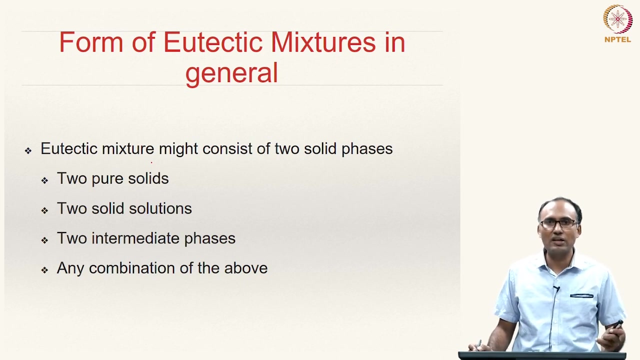 So when we are talking about this, when we have a liquid solution which is reaching eutectic composition at the eutectic temperature, it has to go through this eutectic reaction And the liquid should transform to two solids And, in general, the eutectic mixtures in general. 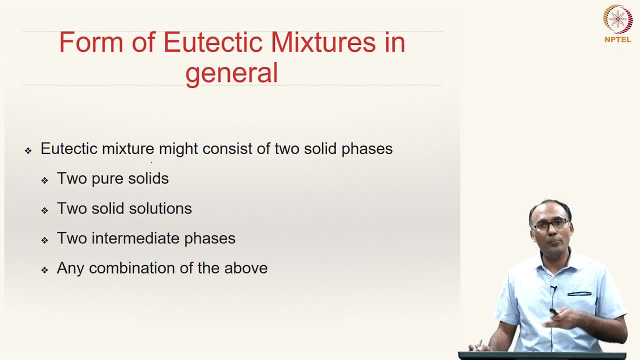 not for only type II alloys. you can also have eutectic mixtures. You can also have eutectic mixtures where you have partial solubility in solid state, and so on. So in general, the eutectic mixture might consist of two solid phases And thus two solid phases. 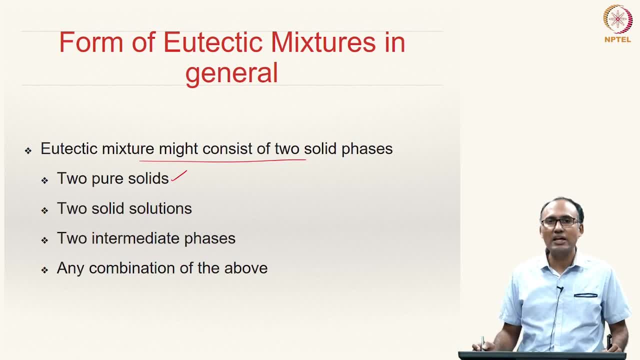 that we are talking about can be two pure solids, like in the case of type II alloy that we have looked at, or two solid solutions, or two intermediate phases, or any combination of the above. You can have one solid, one solid solution, one solid, one intermediate.